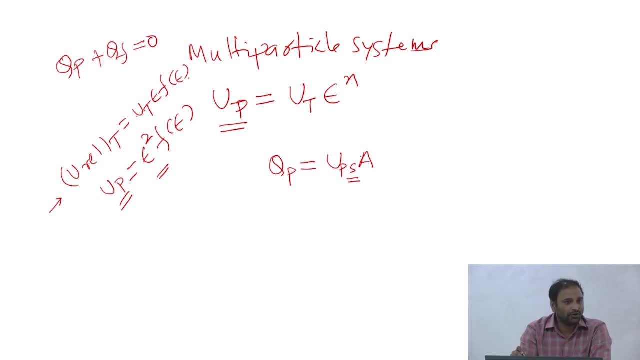 times a, which is the area of cross section that is available for the entire fluid particle system to flow. r. that is equal to u p times 1 minus epsilon, because you know times a, of course. right, there is a as well. Only thing I have done is I have only taken the 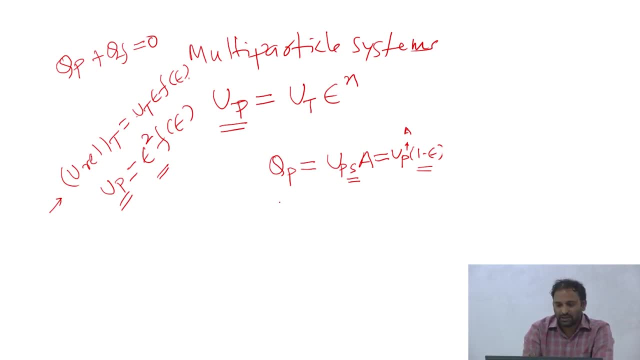 area that is available for the particles to flow right. Similarly, I can write u q f, which is the volumetric flow rate of the liquid, as u fluid superficial s 0.. So here it is a specific fluid which will be a place for the particles. 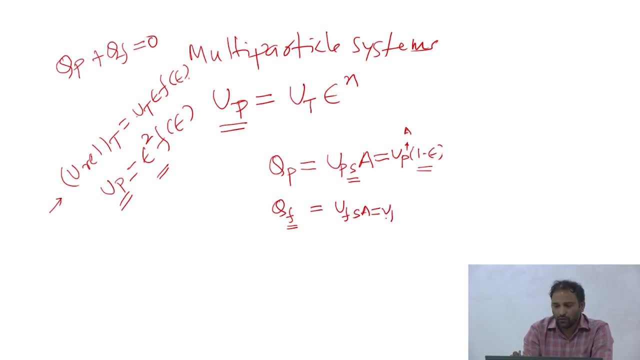 times a, that is equal to u fluid times a, into epsilon, right? This basically comes from the couple of definitions of: you know the superficial velocities and the actual velocities, right? Then we went on to say that you know this f of epsilon is a function which is typically 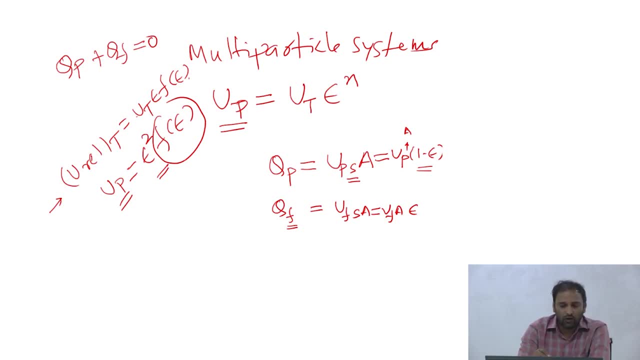 less than 1 and there are different models that people have proposed and, according to one of the you know models, your f of epsilon was, you know, epsilon to the power 2.5 right. we derived that, therefore, your u p comes out to be epsilon to the power of 4.5 and. 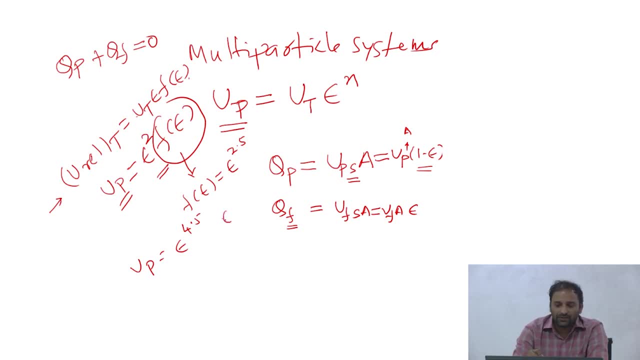 we said, you know this is typically applicable, for you know your epsilon, which is of the order of 0.9, or you know your phi, of the order of about 10 percentage, you know, or a 0.1 percentage. right, And there are lot people have done lot of. 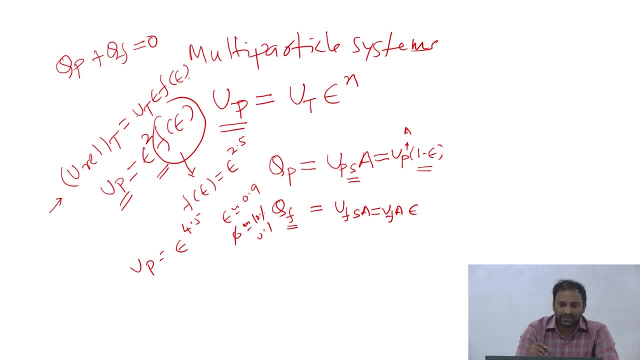 experiments to kind of verify some of these things. and I said that this value of n depends on depends on the kind of condition that you are working with, right, Newton's law, Newton's regime, you know, Stokes regime and things like that. There is a very famous equation: 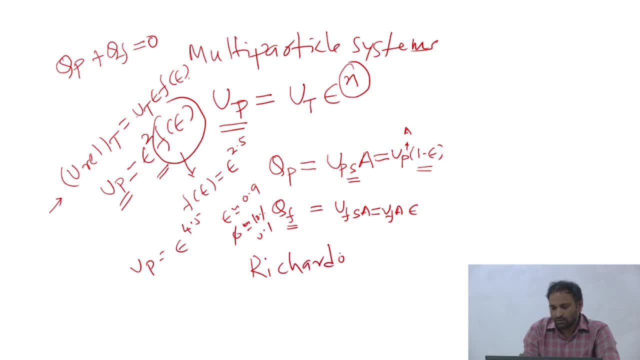 which is what is called as a Richardson Zakai, I think, equation, in which what people did is: they did a lot of experiments on, you know, hindered settling conditions, and they did. they worked with lot of particles of different types, And then they kind of showed that this exponent n is 4.65. ok, though, according to theory it. 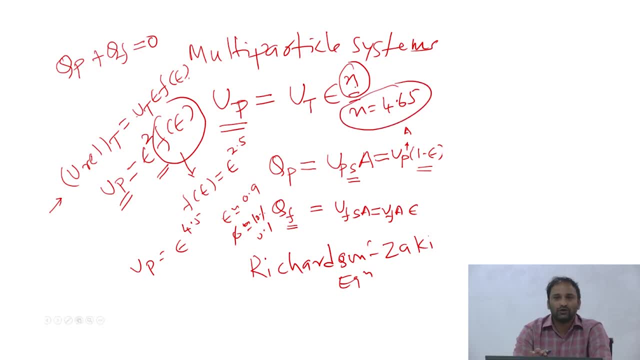 should be about 4.5 and experimentally, people have shown that, you know, this value is typically slightly higher and that which is about 4.65. ok, And other thing that we did was we started talking about u p s by u t. ok, that is a settling. 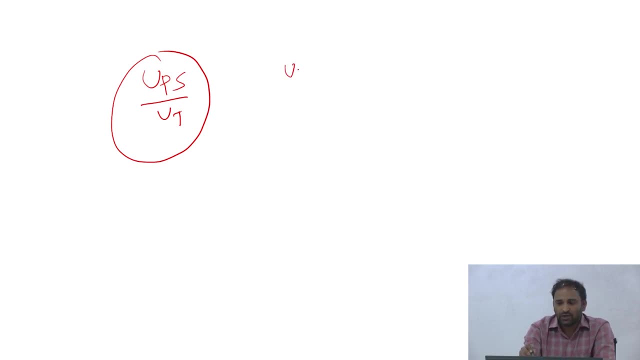 flux, ok, non-dimensional settling flux. and the way we did that was your u p is, you know, epsilon to the power of n times. right u t right, ok, And therefore your u p s, you know this, which is the set: the particle settling velocity, but the superficial velocity, right. 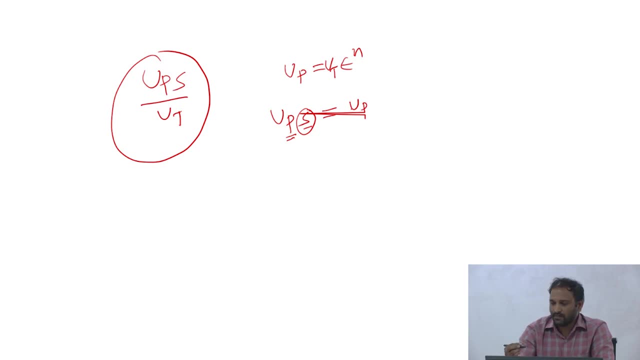 goes as u p times 1 minus. let me just quickly do that. ok, It goes as u p times 1 minus epsilon, right? Therefore your u p s is going to be u t into epsilon 1 minus epsilon, into epsilon power n, right? And we said: if you were to plot this, ok. So 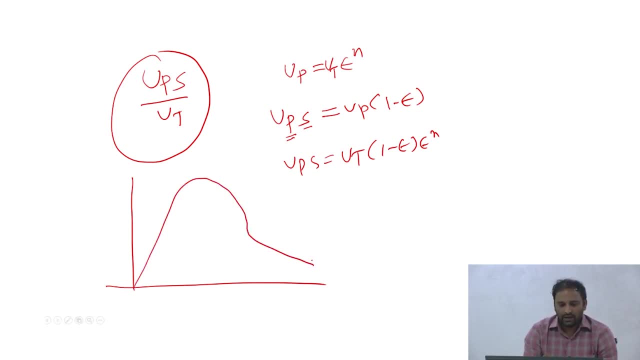 would. the function would go something like: that is what I had mentioned. ok, This is actually plot of u p s by u t versus 1 minus epsilon. I did a mistake in the last class. it is not epsilon, it is 1 minus epsilon. It turns out I can get this point and this point just by 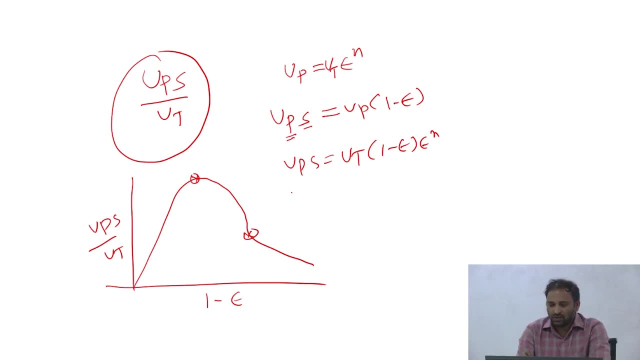 differentiating this one you know couple of times right. So if I do that, so if I take this u p s by u t and if I differentiate it once, ok, d by d epsilon, if you do it, ok, What I will do is I will get this as 1 minus epsilon into. 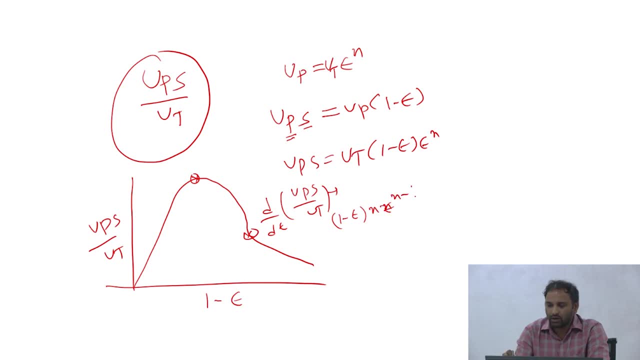 n into n minus epsilon. So I will get this as 1 minus epsilon into n into n minus epsilon. So I will get this epsilon power n minus 1, plus of minus 1, into epsilon power. n is equal to 0 if I equate that as 0. Therefore, if I work this out, I would basically get an. 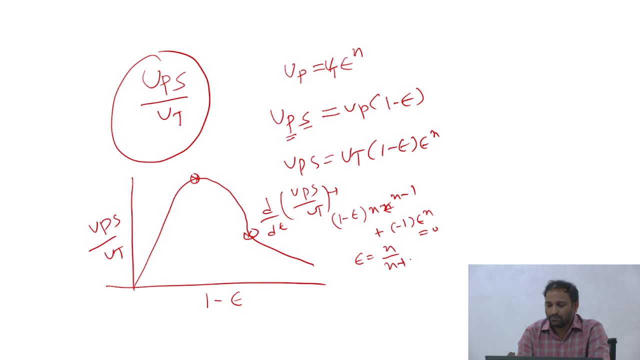 expression for epsilon as n divided by n plus 1. that is your, this point, ok, And if I do the double derivative, and if I do it basically, it come you know, this particular point comes across to be n minus 1 divided by n plus 1. ok, And this is this particular plot, is you? 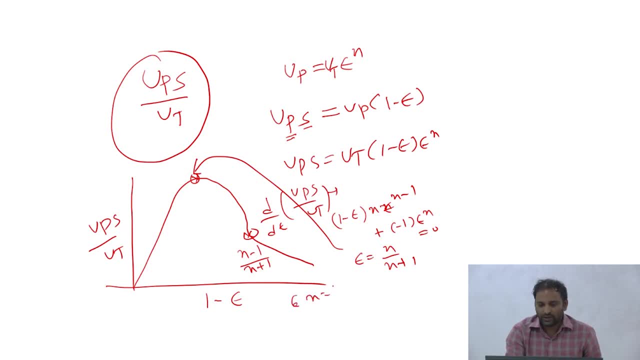 know what I have drawn is for epsilon. sorry, n is equal to 4.65. that is the Richardson Zacche equation. ok, And it turns out, you know, this particular point corresponds to 0.177 and this point corresponds to 0.35.. That means, if I have 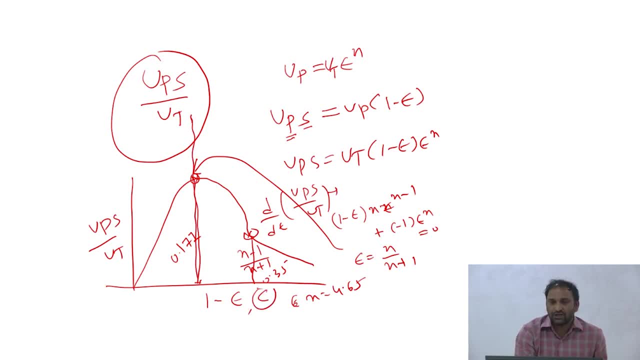 you know this is 1 minus epsilon, or it is in, it is a concentration, right, or you can think about this as a particle fraction. And if your particle concentration is less than 0.177, you know you will see some kind of settling behavior in your system. And then you know. 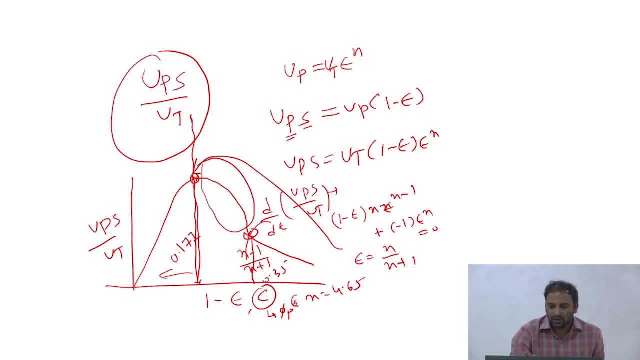 you know of course there is some region where you see some other settling region and you know So. so, basically, depending upon the initial concentration that you work with the settling, if you were to do this batch settling experiments, you will see different behavior that I discussed in the last class right. There is a type 1. 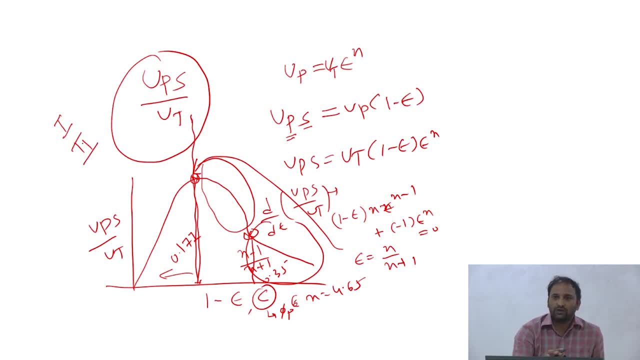 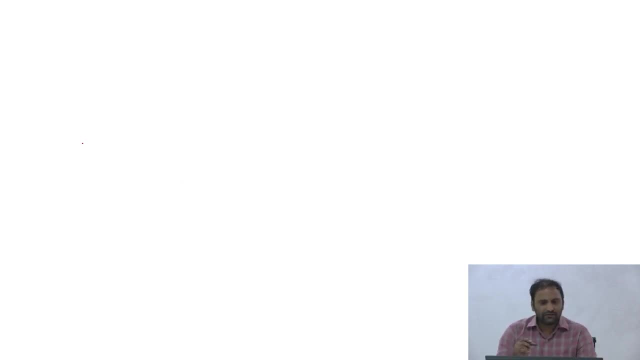 settling or type 2 settling, or something very different from the these two. everything depends on the initial concentration of the you know particle that you work with, ok, And in the case of so, the other point that I wanted to mention is What is called, as you know there are. when you do the settling experiments, you will always 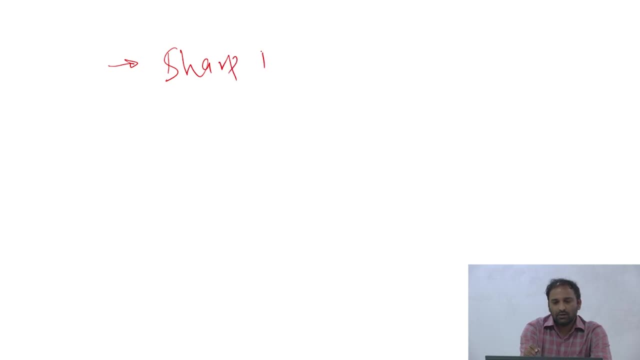 have sharp interfaces. ok, That is what I kind of showed in those batch settling. you know experiments right. So that means I could have a case where you know I have a uniform dispersion. to begin with everywhere the particle concentration is the same. but then you know. 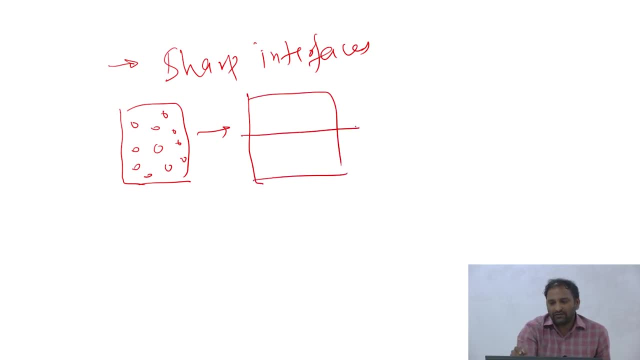 at some point in time. you would have a case where I have an interface- ok, And I could have a case where I have a clear fluid at the top and you know all the particles at the bottom, or, in general, I could have a case where the particle concentration is less here. 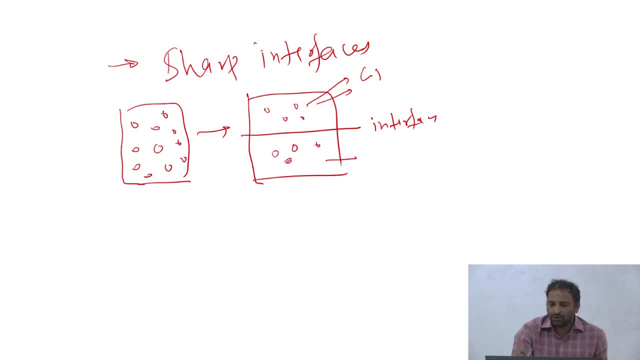 concentration could be C 1 here and the particle concentration could be bit more here, right? So in such a case I can have an settling velocity associated with each of these phases. ok, it, this could be U P 1, you can take it as regime 1 or 2, and in this case you know. 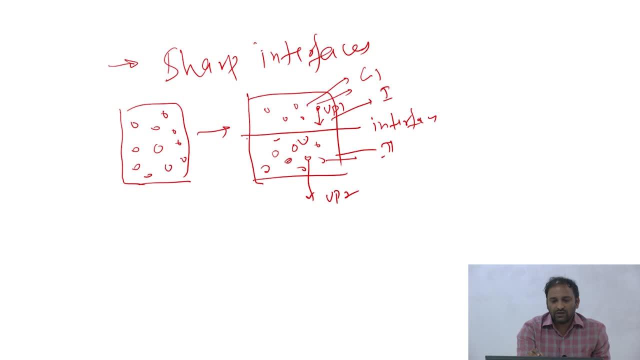 the settling velocity is going to be U P 2.. And if the, if your interface is moving in down with the velocity U int, that is the interface velocity and I said, you can think about writing a simple mass balance which basically is U P 1 minus U interface, multiplied by your concentration. 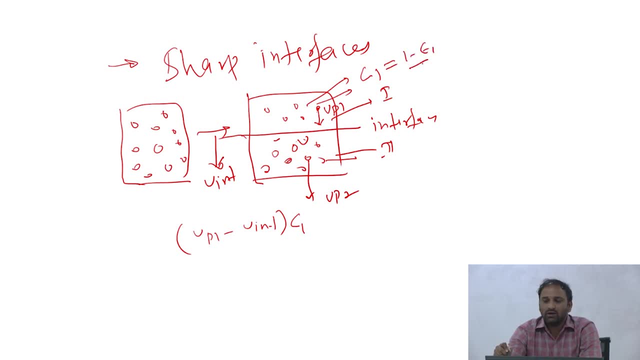 concentration. C 1 in this case is 1 minus epsilon 1.. You are basically expressing this in terms of the you know void fraction right should be equal to U P 2 minus U int into C 2 right. If you work it out, it turns out. you know this. 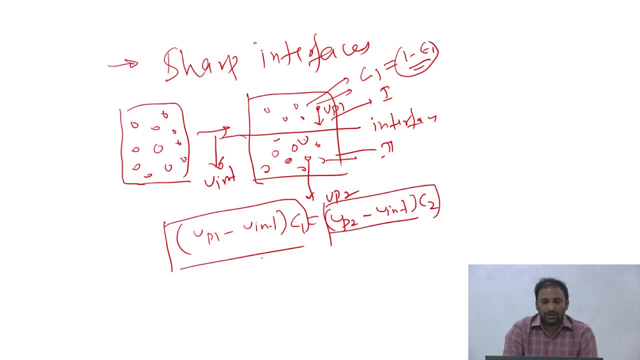 basically will have Points of mass per second, ok, because this is, you know, meter per second, right, and this is your concentration volume fraction. of course I can have the area multiplied on both sides, right? So basically this is a, is a mass balance, which basically is telling you that, if you 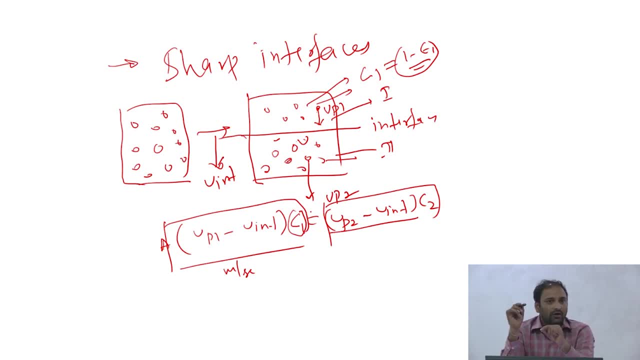 want to have a clear interface. whatever the number of particles or the concentration of the particle, that that that will reach the interface, the same number of particles have to go out, ok, So so, if you work it out, your U I P 1 is not the same, So your U I int becomes U P 1 C 1 minus U. 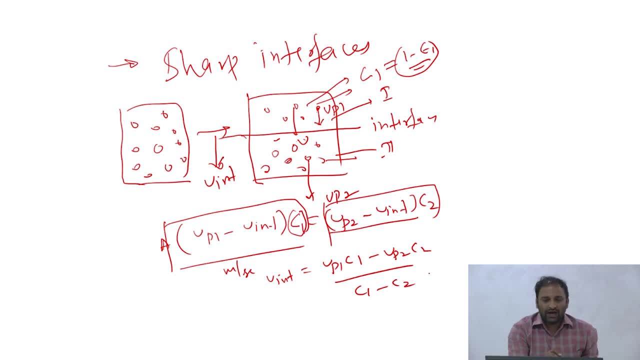 P 2, C 2 divided by C 1 minus C 2.. If I have a case where I have a clear fluid here and then all the particles are in the, you know, in the bottom region regime, So one of the concentration is going to be 0, right? if you say the C 1 is 0, that is a in the top regime. 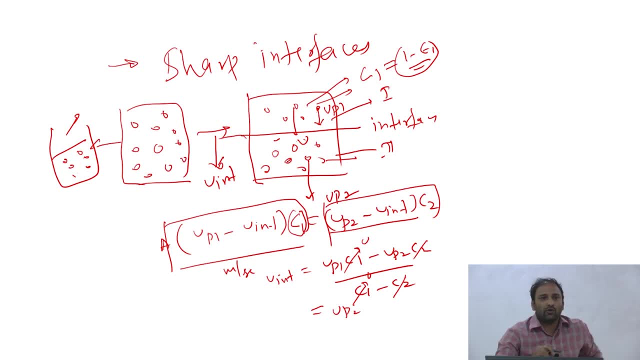 So basically this, this gets cancelled, you basically get U P 2 itself, right. So therefore, when you do this settling experiments, you know when you are following the interface velocity, right, which is basically you know. I said that right, if you have different interfaces, there could. 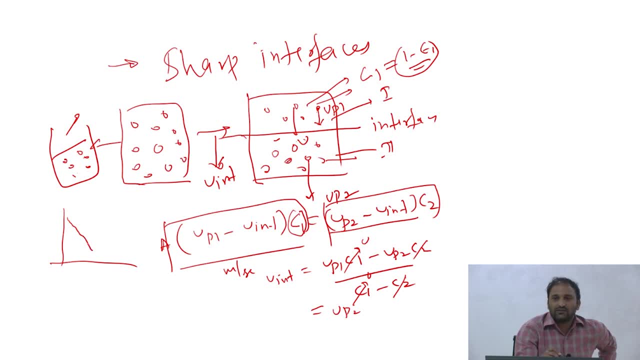 be a case where some interfaces are basically, you know, falling as a function of time. there could be cases where the interface is, you know, rising as a function of time. All I need to do is get this slope that is you are plotting, you know, height versus time. 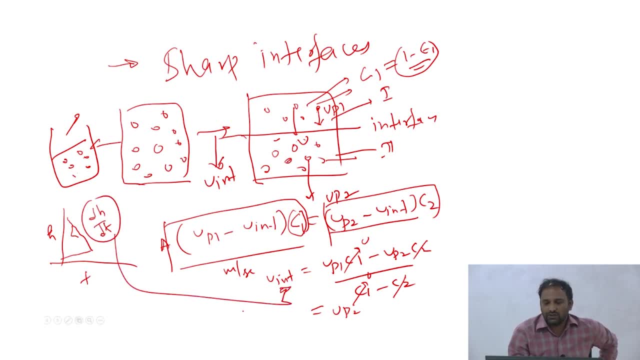 I get this d h by d t. that is basically my interface velocity and from that I have a way of calculating the settling velocity. ok, So maybe we will stop here at this point. So we have talked about you know different things in the in the previous lectures, right? 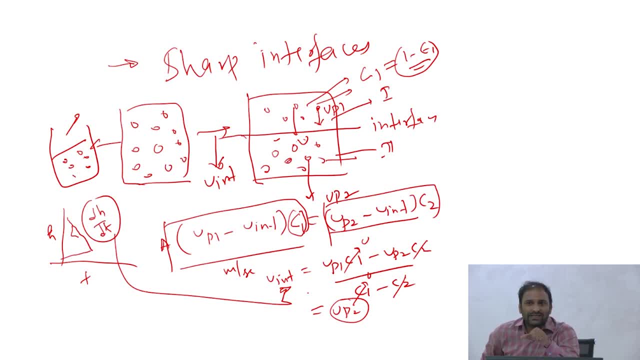 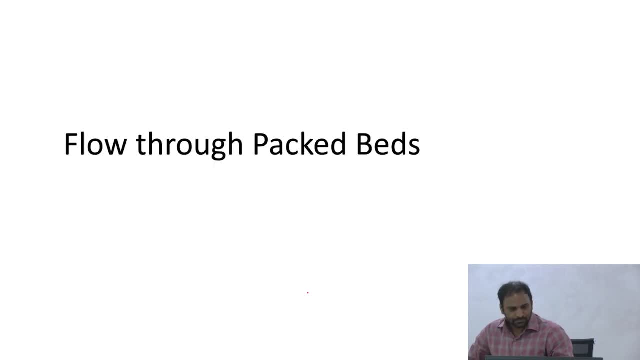 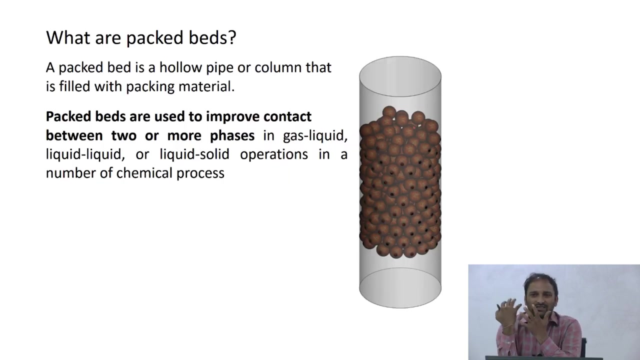 we talked about settling of single particles, then we talked about how do we extend that to an aggregate of particles and then again extension of the similar concept to cases where we have multiple particle systems, right. So now we will talk about a concept called flow through packed beds. ok, And in a sense packed beds are kind of. it is a simple concept. 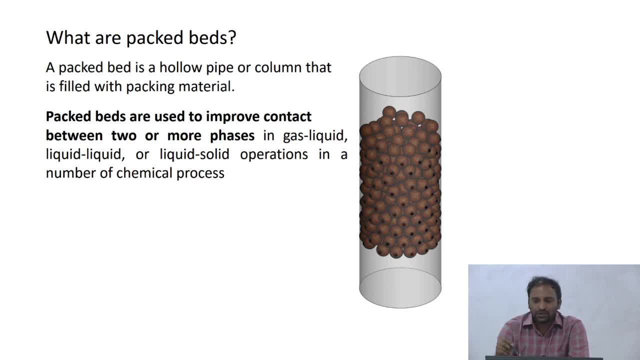 you know, what do you basically mean by packed bed is you basically have a column- it could be a pipe, it could be you know, a container, right, and this column is basically filled with. this is your column, this is your packing material. ok, Now, I had mentioned in you know, a few lectures ago that the reason why the packed beds are 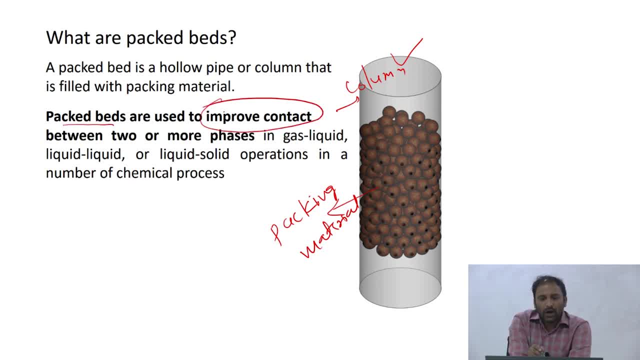 used are Because they want, you know, they provide us a way of improving the contact between two or more phases. ok, I could have a case you know, for example. say that you know I have a, say, a simple pipe, hollow pipe, and in which you know I am want to send two liquids. ok, 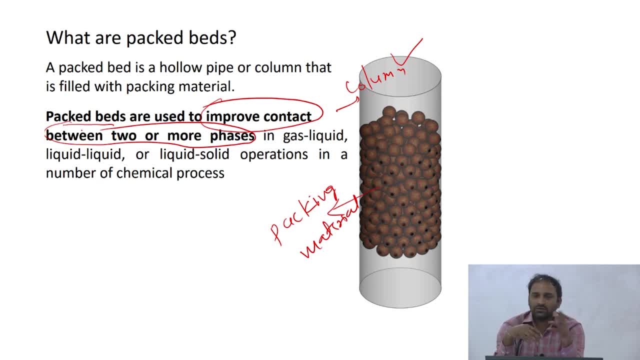 Like say, you know, maybe some methane or you know some liquid and a gas, for example, if I want to ensure a proper contact between the two, if I were to have a simple pipe without any of these abstraction, you know, So there is no proper contact between the two phases, right, two fluid phases, ok. So therefore, 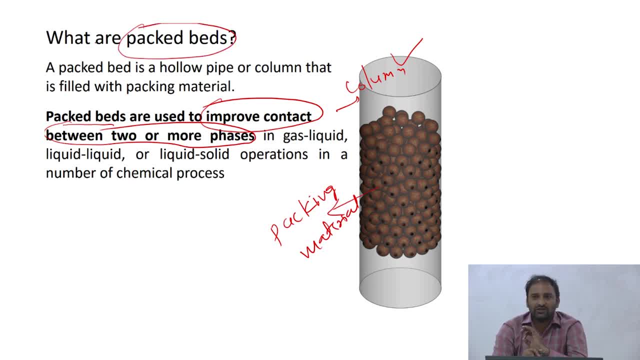 the one of the main advantages of using this packed beds is you know they essentially ensure that if you have a two phase or three phase, you know systems. they give you a way of improving the contact between different phases. ok, And people typically use this for the cases where 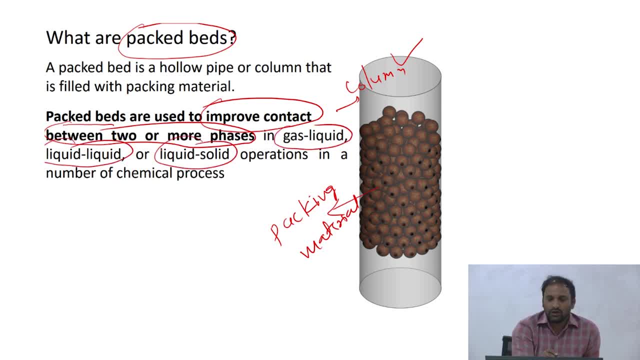 there is a gas liquid operation or a liquid liquid or a liquid solid, depending upon. you know there are lot of cases in chemical industries where you come across you know different. you know fluids that are going to be, you know you want them to be in contact, either liquid. 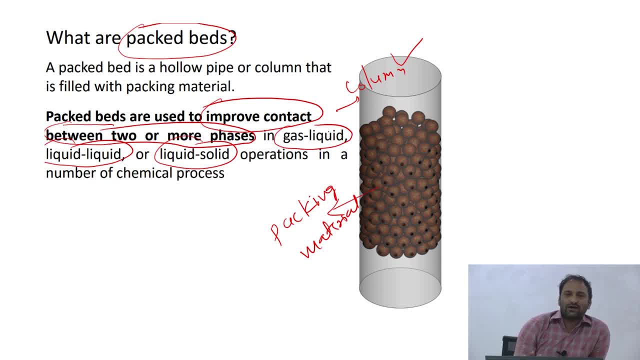 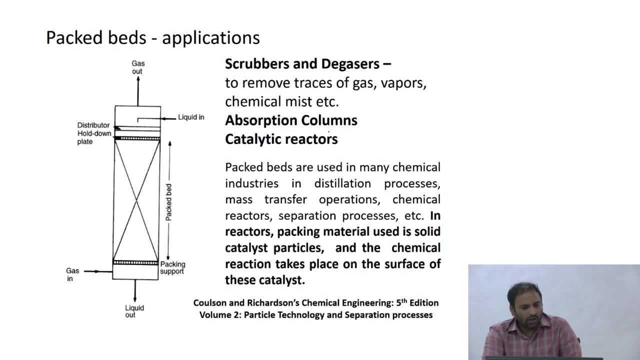 liquid, liquid solid or gas solid. So in such cases, people make use of these devices to ensure that, you know, there is a proper contact between the different, between different phases. ok Now, so this is again a schematic that I picked up. this is an example. 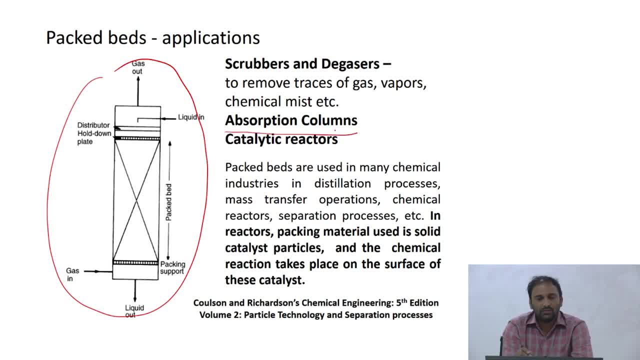 of a case where people have this is an, an absorption column. ok, Again, typically what you will have is: you know, some packing material in the pipe, there is some liquid that is coming in, there could be some gas that is coming out. you know, if your objective is to either. 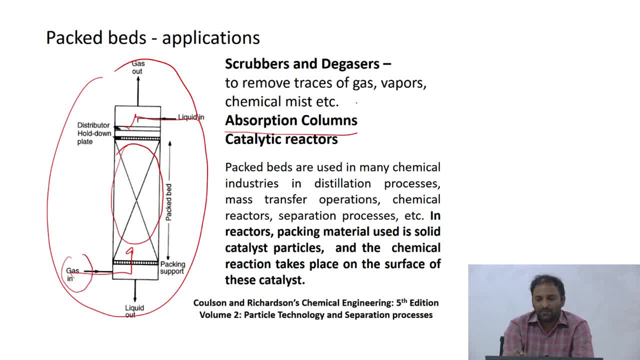 you know, take out if you have a. if there is a gas, for example, if the gas has some trace amount of chemical, for example mist, you know, or if there is some, for example, if I want to have a clean gas that I want to come out, ok, If there is some unwanted gas that you. 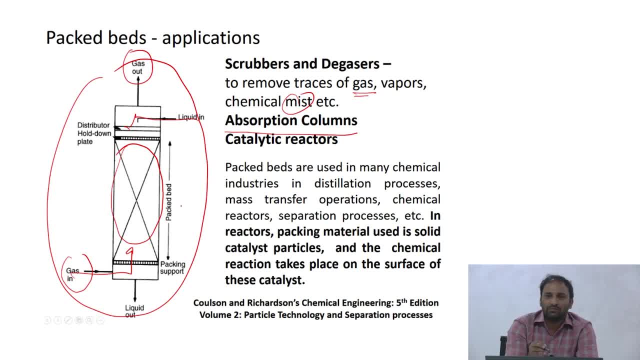 want to separate out, ok, One of the best way to doing this would be use of this packed bed. ok, let it pass through the pass up through the column and then, you know, use an appropriate liquid which basically takes out this unwanted, you know- material. ok, and it comes out at the bottom and again, 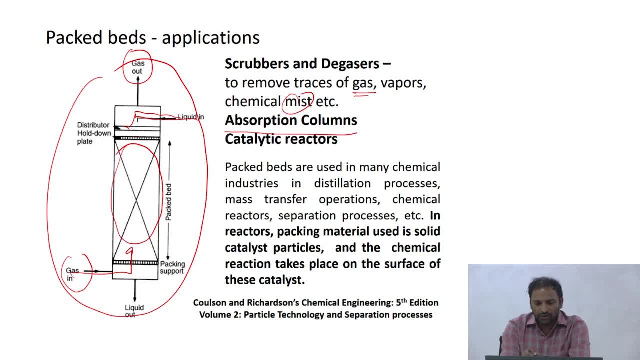 you can, you know, subject to whatever purification that you want to do, ok. And people use them for the scrubbing or degassing operations. ok, which is to remove traces of gas vapors or chemical mist Absorption column. people use it for, you know, catalytic reactors. ok, if you. 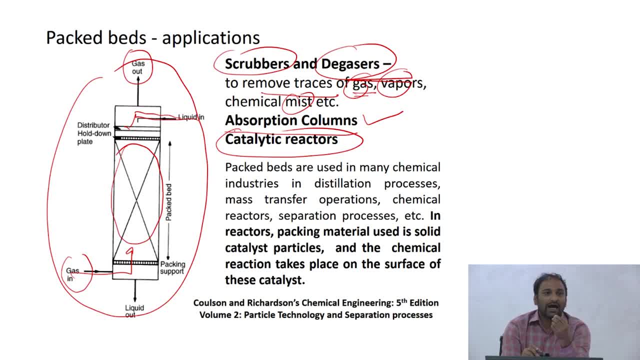 really want to. If you want to have a particular reaction that I want to occur over a solid surface, ok. The best way of doing this would be, again, you pack them into these columns, ok, and as you let either a liquid or a gas through this column, on the surface of this catalyst, you. 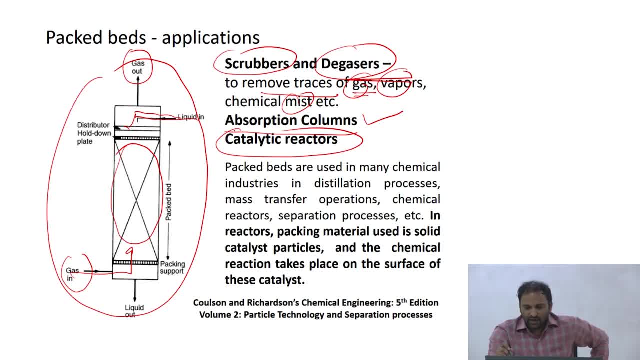 know some reaction may occur, right? So yeah, as I said, right, they are used for distillation operations. a lot of mass transfer operation in absorption is one example. I talked about chemical reactors, separators, ok. So so these have very wide applications, ok, And I will. 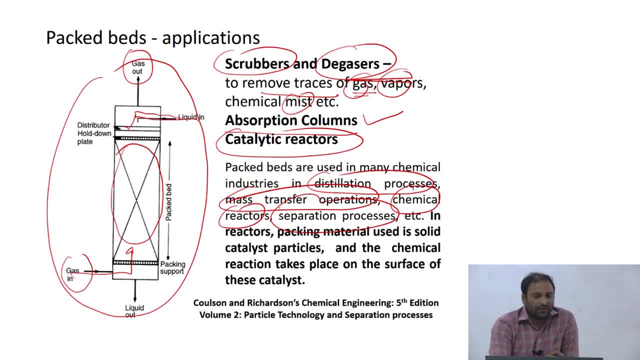 talk about that later. ok, and you will have couple of experiments in the in the next semester to look at. you know different aspects of flow through packed beds. ok, So now before we go to. So the reason why we are interested in a packed column is because 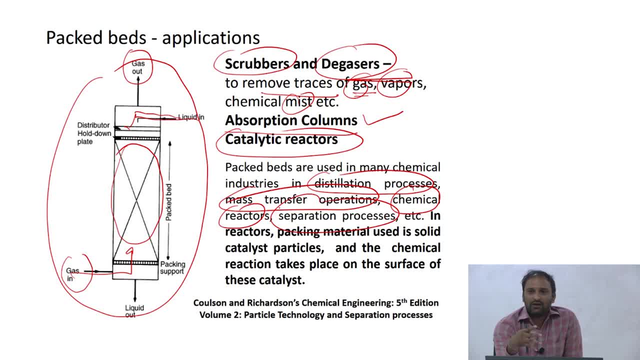 like we talked about pressure drop in a in a pipe right Now, that now, if you have a pipe that is filled with you know particles, right Again now, the fact that you know there is much more obstruction for the liquid to flow through, Your delta p is going to be much, much larger compared to the you know case of flow through. 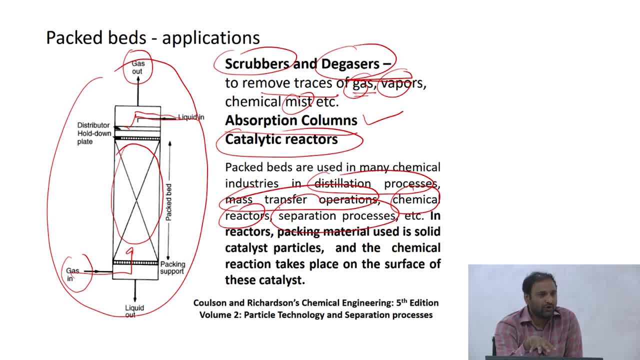 pipe right. So so the ultimate aim of the some other thing that we are going to discuss is to look at how do we think about pressure drop through this such system. Then we are going to think about some ways of analyzing. you know, flow through the packed bed and you 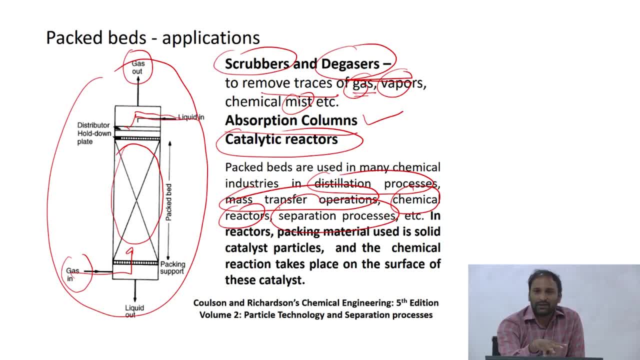 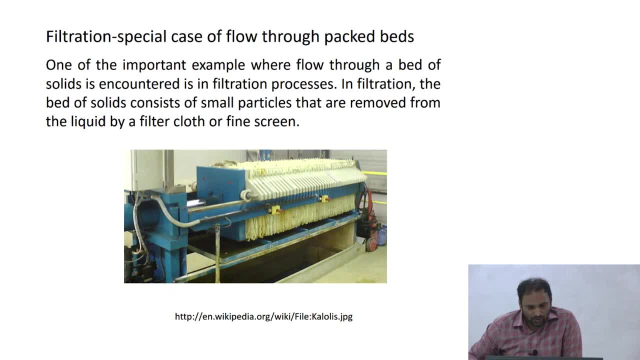 know how do we kind of correlate the pressure drop to different parameters, like you know the structure of the packing, you know flow of the flow, rate of the liquid, and you know few things like that is what we are going to do, ok, So, so it turns out that you know. 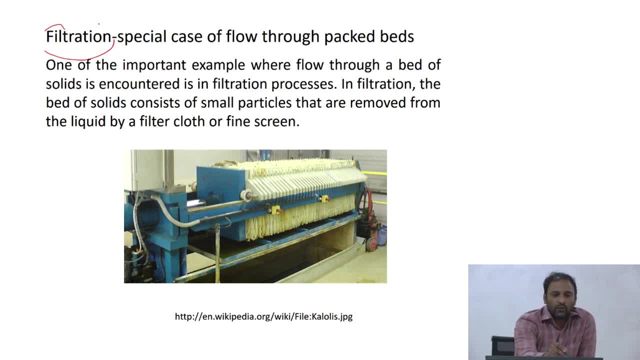 you see A particular operation called filtration, ok, which is some kind of a. it is a special case of flow through packed bed, right Again, filtration, one of the simplest thing that you can think about. you know, when people do this coffee or tea at home, right when you, when you strain. 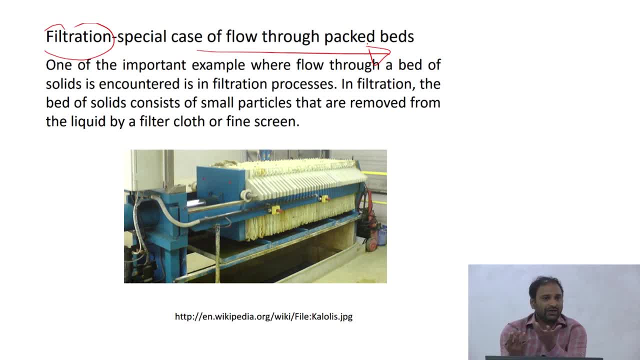 the coffee or or the tea. ok, On the you know strainer: right, you have some solid bed. that is ok. Initially it is a, it is a clean, you know cloth or something like that. at some point in time, you know, as you start straining it, you have a bed of solid. that form right. 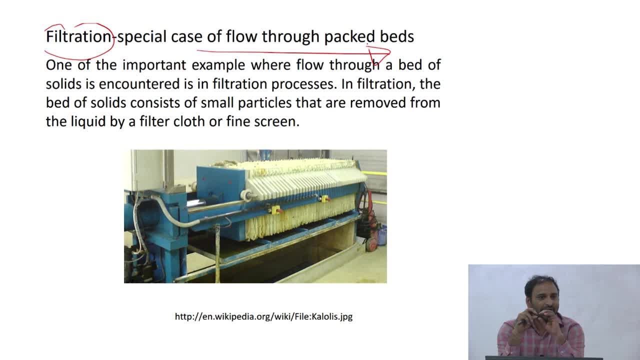 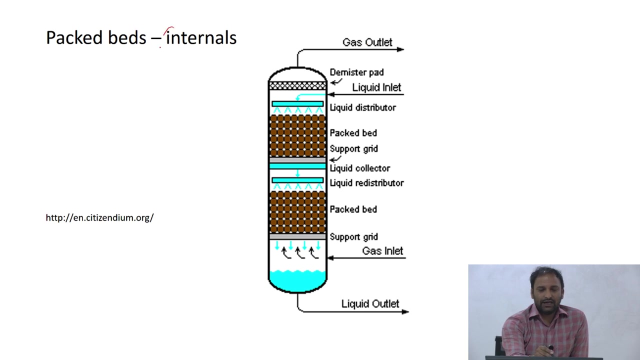 So ultimately, you know, the liquid starts flowing. 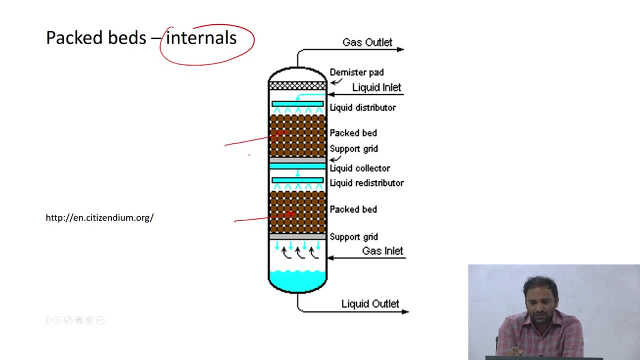 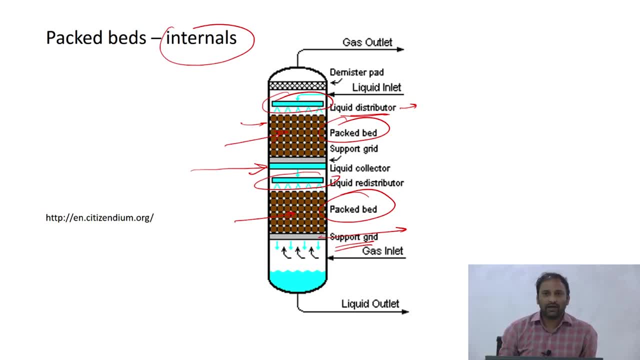 you know, you know this liquid takes some preferential paths. ok, and these are the least resistance path. ok, One of the way to avoid that would be you put in this liquid collector. ok, The job of this liquid collector is it basically collect the liquid as coming out down the 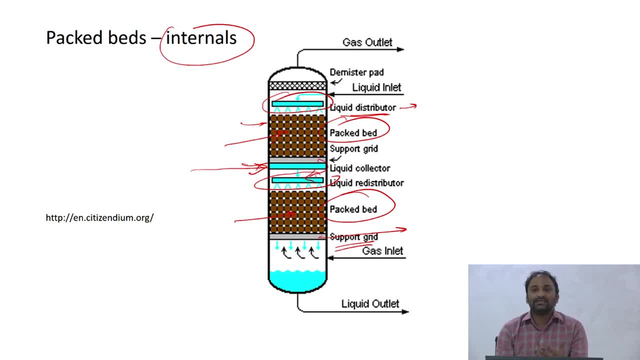 back column and then, you know, it kind of feeds it to a liquid redistributor. ok, So these operations, you know these kind of internals are really required to ensure that the flow rate across the different cross sections of the bed is kind of uniform. So you know, 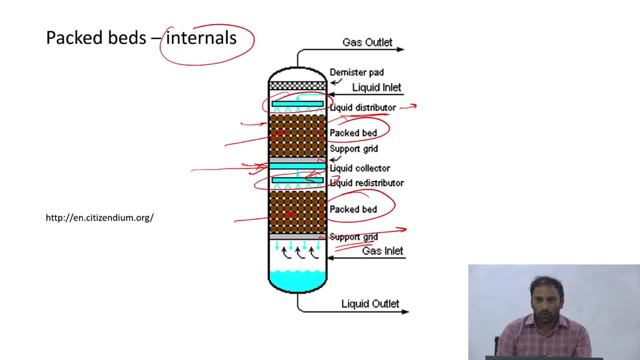 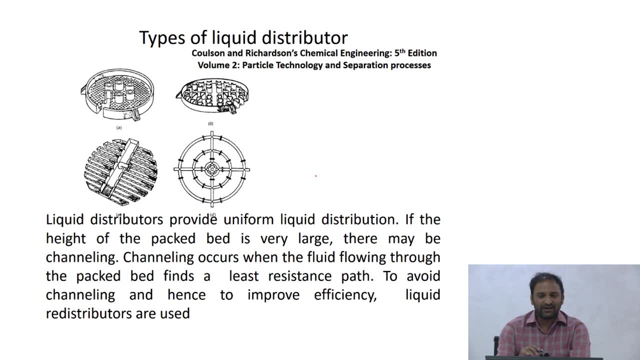 there is a proper contact between the fluids that you are trying to work with. ok, So this is a different kind of liquid distributor, as I was mentioning. liquid distributor basically provide uniform distribution of liquid and, as I said, if the height of the packed bed is very, very large, there may be something called as a channeling. the channeling is what 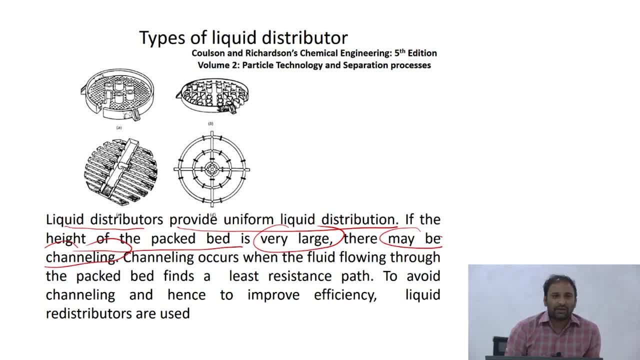 I said, you know when the, when the liquid starts taking some preferential paths, that means there is a larger flow in one region of the packed bed versus the other region. ok, That is when you have what is called as a channeling, and channeling can be avoided if you use these. 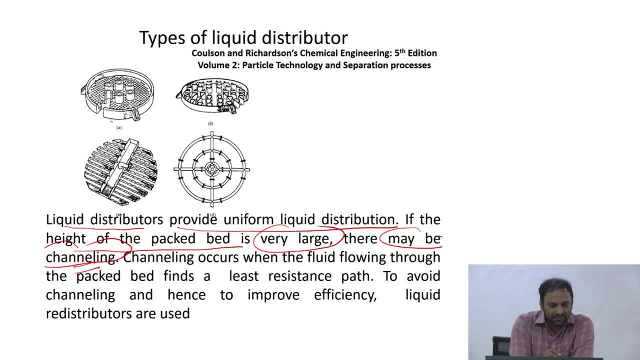 redistributors and things like that. ok, So these are four different types of distributors people use. These are some kind of a porous pipes. ok, This is a pipe through which the liquid is flowing, but you know, there are regions where, you know, I let the liquid into. 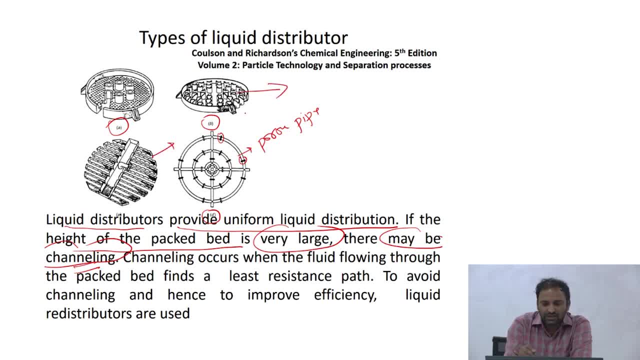 the column. These two, this and this. these are what are called a notch type distributor. ok, If you see this right, there is a wedge kind of thing. right, if you look at these things. So there is a. the construction is something like this: 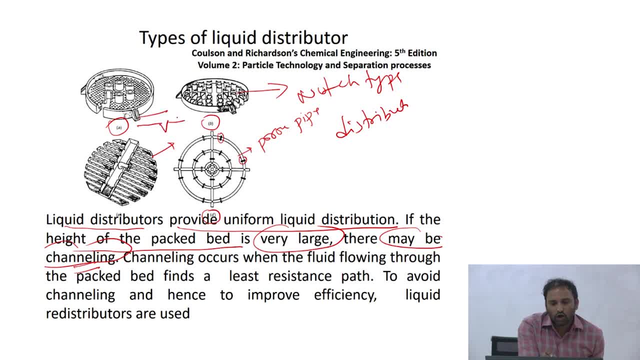 ok, There is a parallel channel like that channel, like that, and then there is a notch, ok, and basically you fill the liquid in this, you know these, you know channels- and then through the notch, the liquid basically comes down. ok, That is the case here and here. ok, 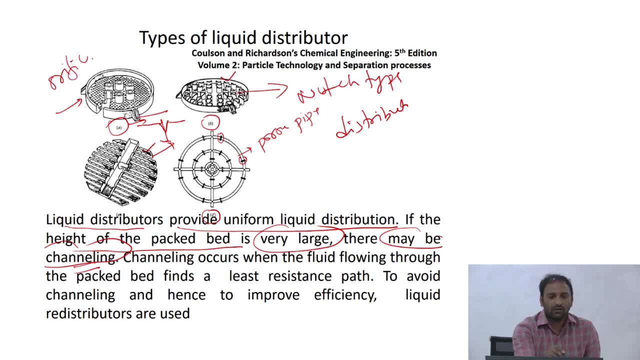 This is an example of what is called a orifice, you know type of distribution, So liquid distributor, which basically has porous- you know porous- openings, right, and then through that the liquid basically flows. ok, So these are what people typically, you know, use and, as I said, right, the objective of this liquid distributor is to ensure that. 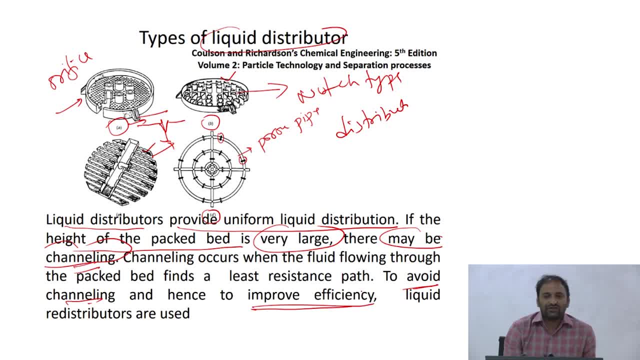 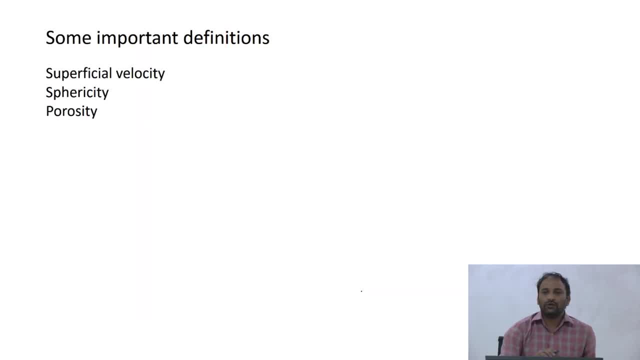 to avoid channeling and to ensure that there is a improved efficiency. right, that is the whole point. Now I just want to define a few terms. ok, First term that we are going to do is something about the porosity or a few alternatives. 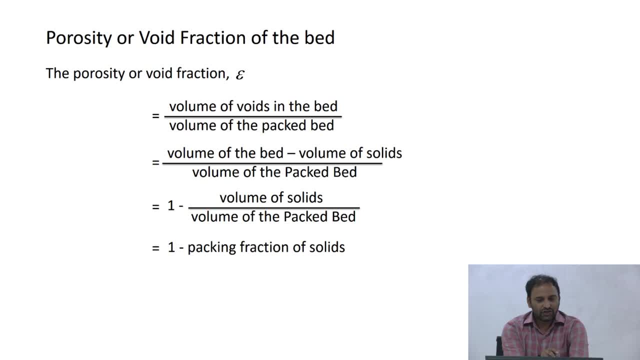 So if you already know this concept, but I still want to do it quickly, ok. So porosity: it is also called as a void fraction. void fraction or porosity, or people, also called as a voidage, is defined as volume of the voids in the bed divided by the volume of the packed. 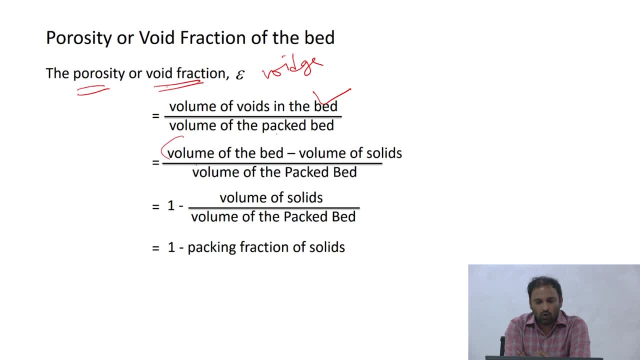 bed And volume of the voids in the bed. I can basically write it as volume of the bed minus volume of the solids right, And therefore I can write this as 1 minus volume of the solids divided by volume of the a packed bed. ok, And volume of the solids divided by volume of the packed bed. we know. 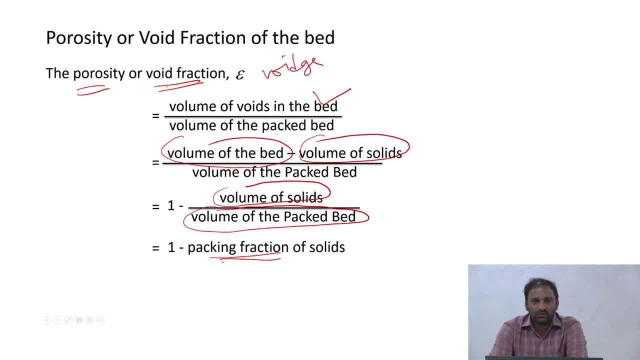 that you know is the a packing fraction of the solid right. So that is a typical definition of. you know the voidage Now. so how do we find voidage in the packed bed? ok, So I say that you know. I have a column. 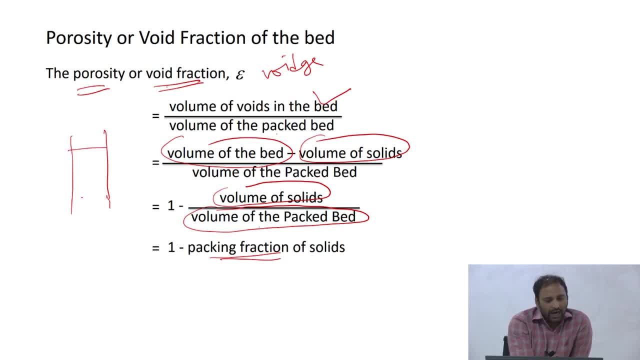 I am going to say that, hey, look, you know, I have a column that is filled with and this is my packed bed. ok, And I want to find out what is a voidage? What do you think is the? you know? can you think of some ways of by which I can measure the void faction? ok, Experimentally. 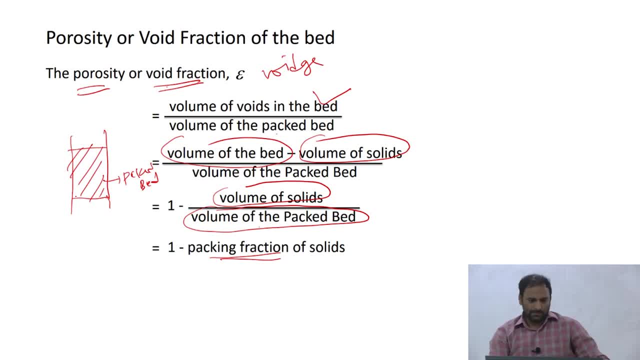 you can think of couple of different simple ways of doing it. ok, What you do is: So you take a empty column, ok, and with a packed bed, what you do is you start going on filling the fluid. ok, you start going on filling the fluid. So, what fluid is going to do is if 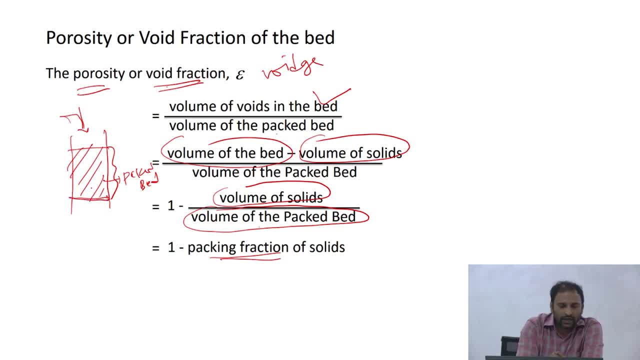 I have a support plate and it will start occupying all the pores in the bed right. the liquid that I am going to add is going to basically occupy all the pores in the fluid. Now what you do is, if you have a some way of collecting that fluid and then measure its volume. ok, 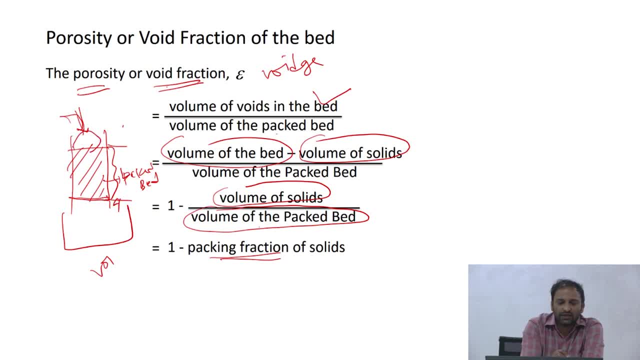 If I know if it is a cylindrical column, if I know the length and the cross sectional area right, I can get the volume of the bed. and if I measure what is the volume that I have collected right. that is one way of doing it. Other ways of doing this would be you. 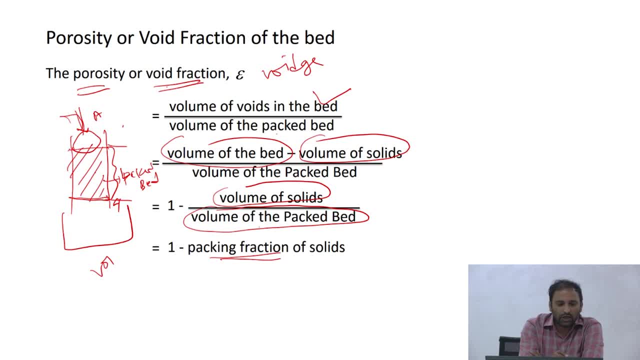 finish up your packed bed experiment and ensure that you know your liquid is basically kind of filled up to the height of the packed bed and we will basically drain the fluid right, So you can different ways of doing. doing that. Now it turns out, the kind of porosity is one of the really important parameters that 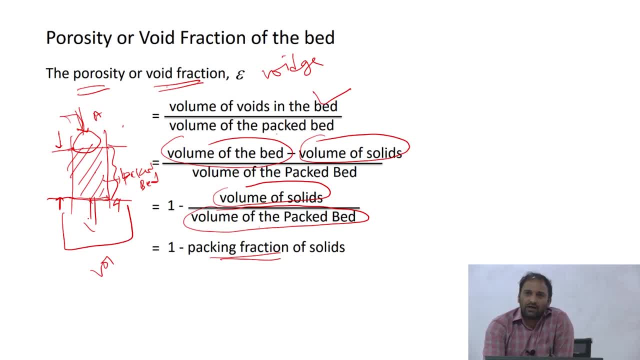 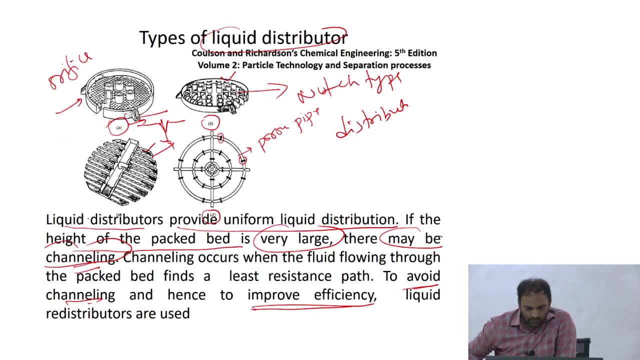 is you know kind of help in the you know kind of achieving. So when I talked about this efficiency- right efficiency, when I when I mean by what I mean by efficiency is that you know if you are able to ensure a better contact between the different phases. that 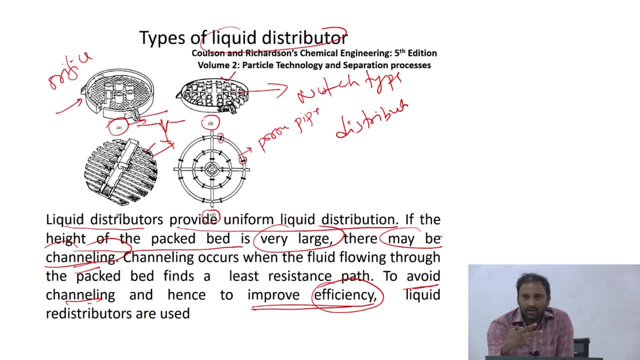 is when you know I can say that you know the efficiency of the operation that I am looking at, whether it is you know reactions or whether it is in a mass transfer operation. that is when that is what I am looking for right To ensure you know improved efficiency, one of the parameter that you can play with. 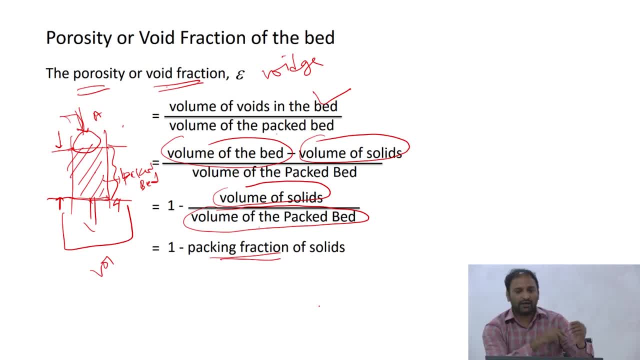 this is porosity. ok, Can you think of ways by which I can play with the porosity of the bed? So I have a packed column is filled with solids. ok, Now what are the different ways by which I can manipulate the porosity in the bed? You can change the. you can change. 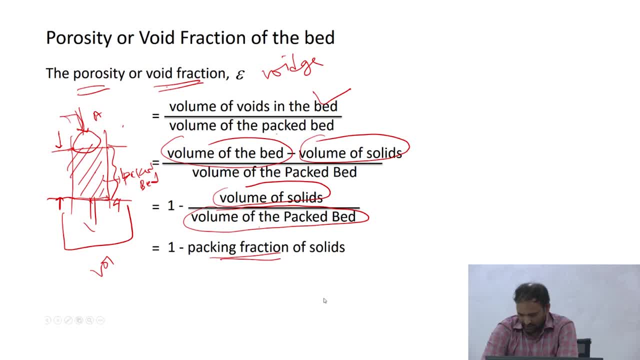 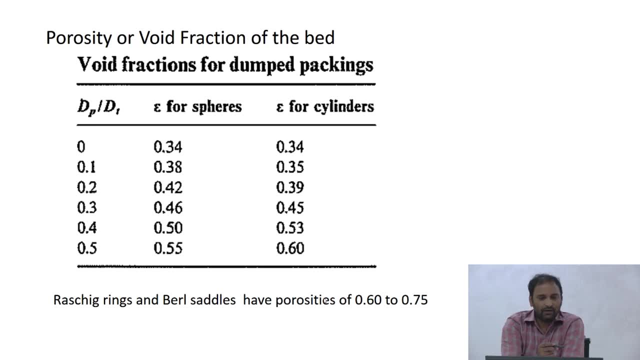 the dimensions of the particle. that is one way of doing it. So he is saying what he is trying to say. let me just go back. ok, So this is a. ok, So what you are seeing here is d p by d t. ok, where d p is the a particle diameter. 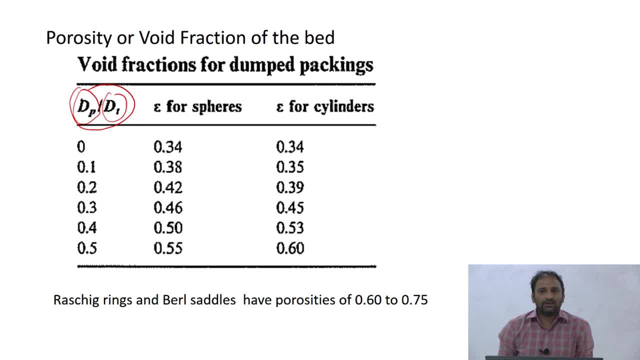 and d? t is the your. you know, if you are have a packed bed, you can think about it as a diameter of the you know column in which the particles are put right Now. so what you are looking at is two columns epsilon for spheres. ok, I am already giving the second hint. ok, this: 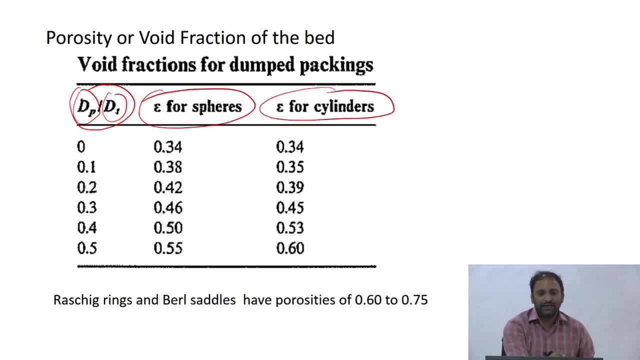 is epsilon for cylinders, ok. Now when you say d p by d t is 0, right. So what does it mean? that basically means that you know, I have a really large column whose diameter is much, much larger than the diameter of the particle that are basically being used. 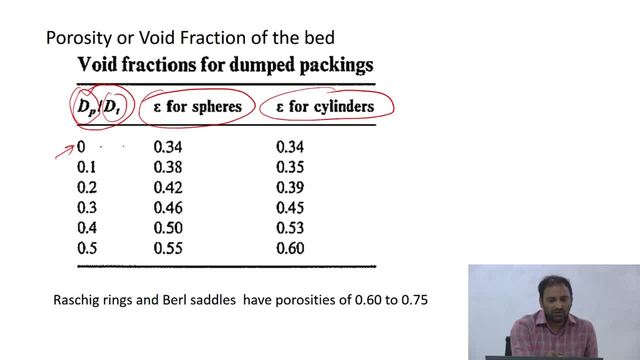 for making the packed bed right. In such a case, your epsilon is 0.0. you know if its 0.0.34 right. this value is very close to very close, to say, if you have some more space, this would be a little bit nicer. 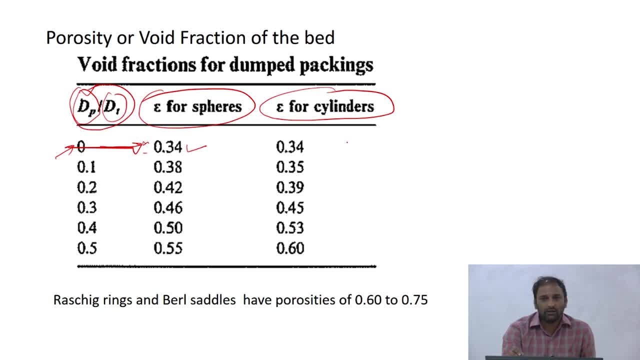 Ok, So let us just say I have a 0.0. this would be very much larger. this value is very close to, very close to, so if you, So if you have a spherical particle, you have something called as a maximum random packing. 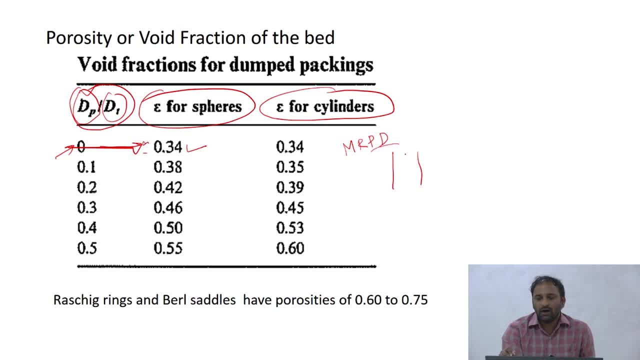 density right. That means if I have a column I pour the particles into the column. if all the particles in the bed, right. if they are arranged in a random, you know configuration right. ok, So it turns out. you know that maximum random packing density is roughly of the order. 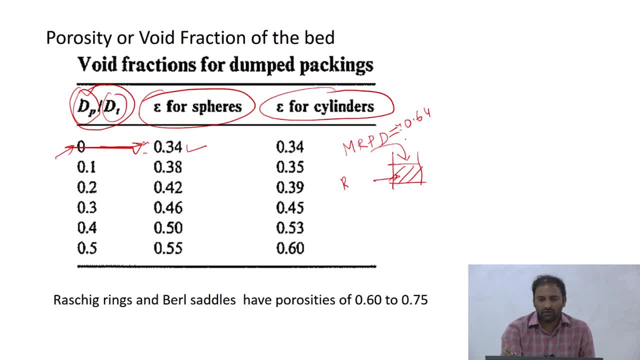 of 0.64, right. Therefore you know the closest that you can get if you really work with. ideally this should be 0.36, ok, but the closest that you get if you really take a very large diameter column and if you put in the particles such that you know the particle diameter is much. 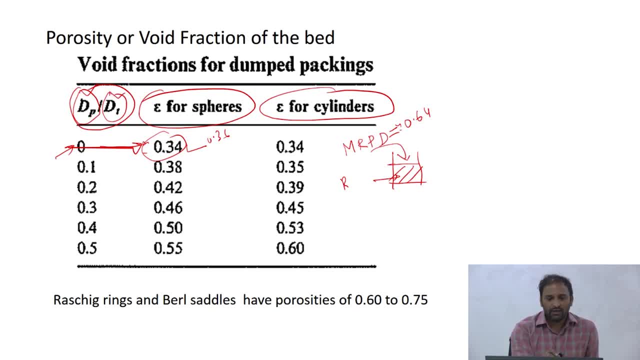 much smaller compared to the diameter of the column right, So you can achieve 0.34, but you can clearly see that if I go on, you know if this, if I go on increasing the diameter of the particle, It turns out. you know this porosity basically. 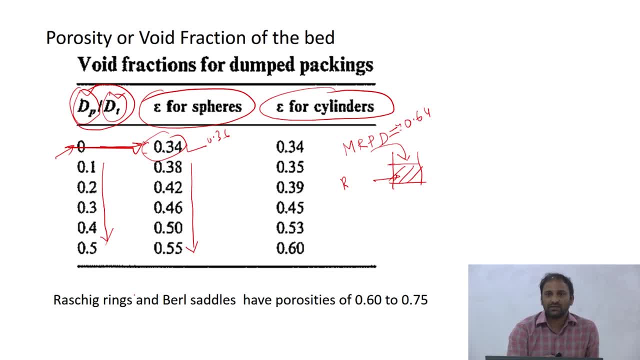 increases, right? does it make sense? because you know, let us think about a simple case, right, If I have a column and I am going to fill in the column with exactly the same, you know diameter particles, right? I am sure you know the, in this case, the. you know the, whatever. 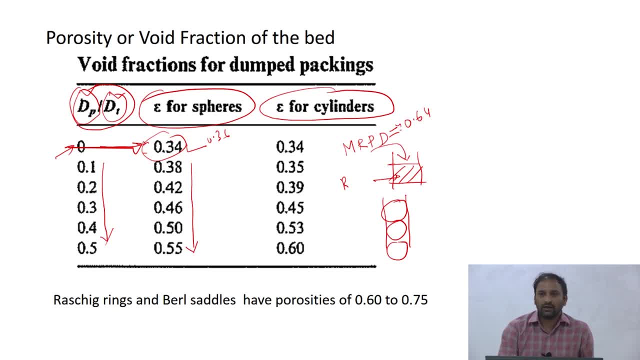 volume that is available for the liquid is very, very little, right? ok, So one of the way of doing this would be: basically, I can play with the diameter of the you know particle to the diameter of the column. but the other ways of doing this would: 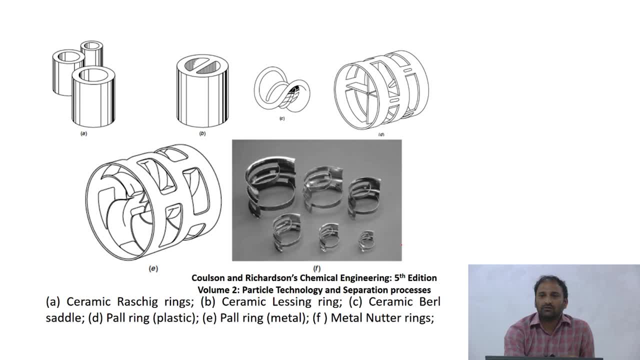 be by using packing materials of different. you know types. ok, Either. so either you can work with regular particles. you can work with, like say, spherical particles or cylindrical particles, for example, or ellipsoids. ok, You can work with particles of you know different. 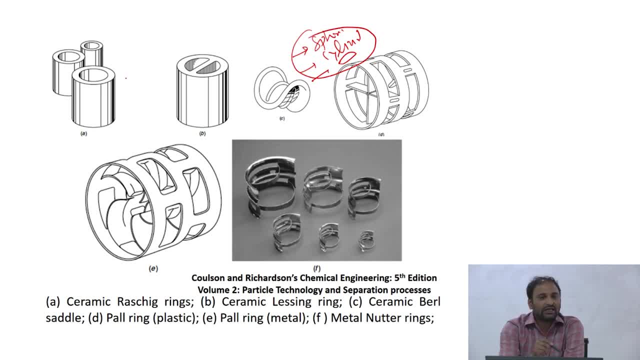 shapes, or people have kind of designed different types of packing material itself. ok, What you are looking at is this: A? ok is a case of what is called as a Raschig rings. these are basically, you know, yeah, go ahead. No, when you say volume of the packed bed, ok, this is the volume of. 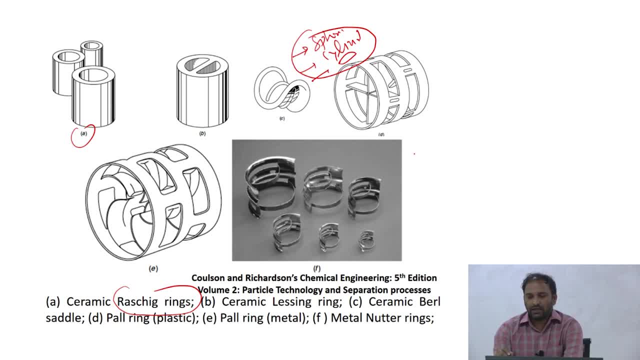 the. So if I have a like, say, say that I have a container, a cylindrical pipe, say that you know my, the packing that I have filled it is up to say length l, for example, ok. And if the diameter is d, right, right that you know pi d square by 4 times l is your volume right. 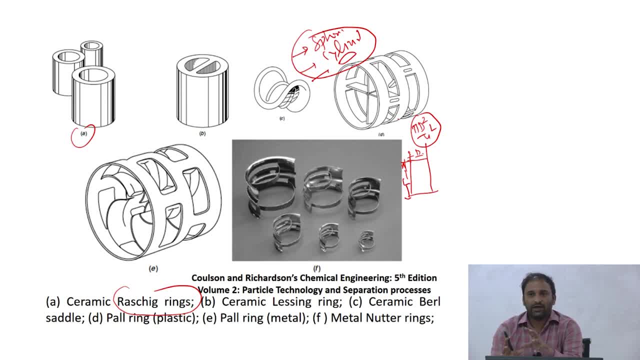 that is the volume of the packed bed. for me, ok, It is not just the volume of the, just the packing itself, and I say volume of the packed bed is So, therefore, so in the, in the example that we saw. So what I can do is I can take a column of some dimension and 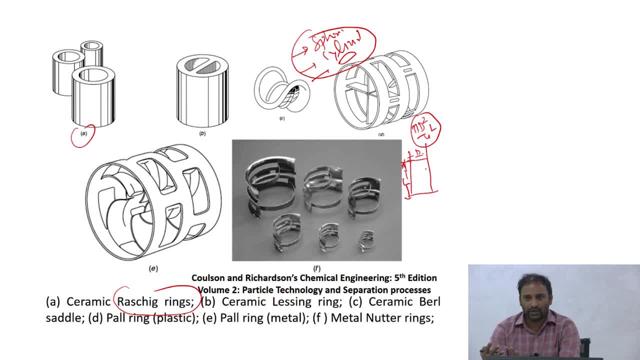 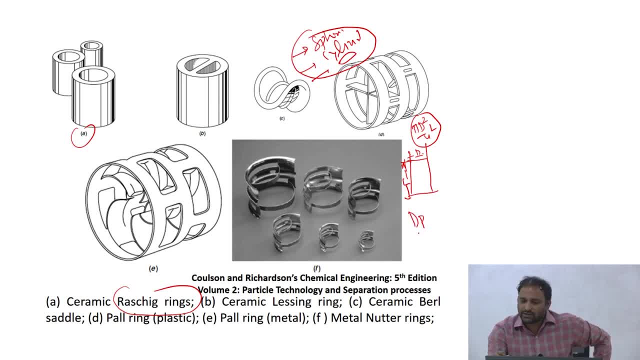 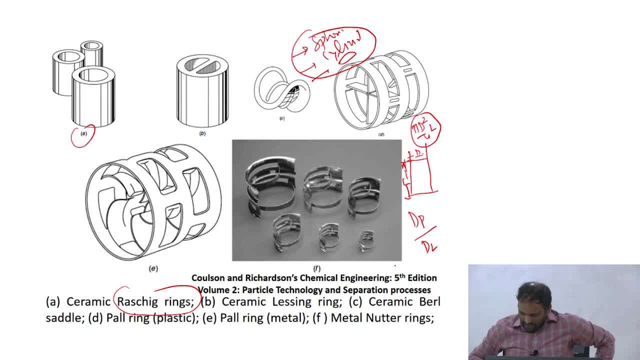 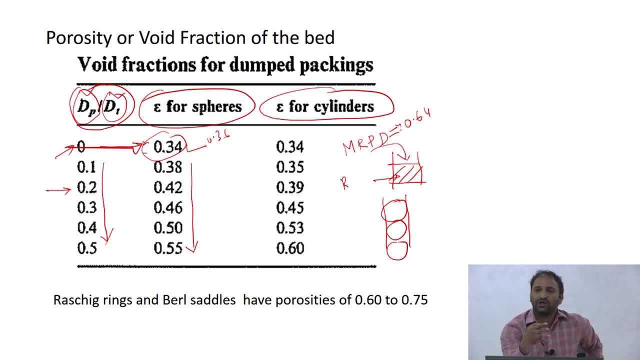 I think so basically no, what this basically tells you. you know, as long as, if you were to do you, you work with any combination of. you know your particle and the, you know the column. So as long as you know, this is actually Here, Anyway. 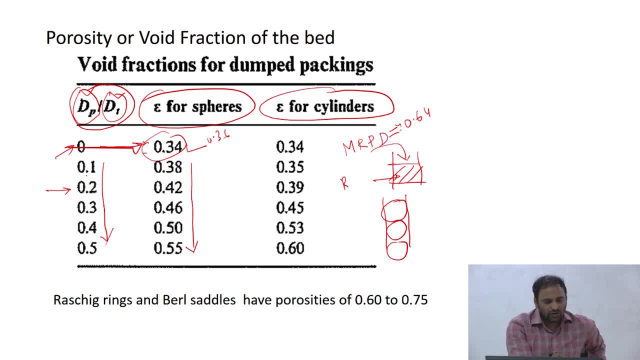 I have taken from one of the books. ok, So the idea is, as long as you maintain this ratio, your the value would be typically close to 0.64.. I mean, you know, or the other way of doing this would be say that, you know, I have like, say, a column which is like, say, 100 centimeter. 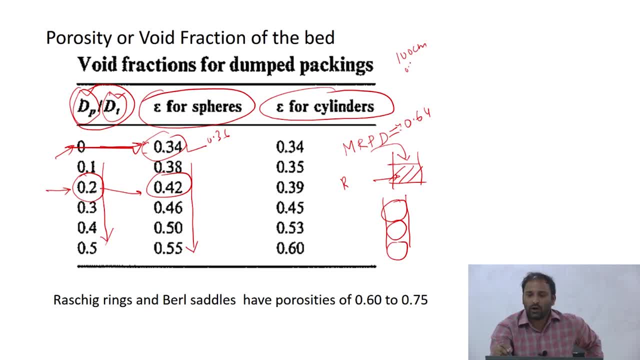 diameter. say that I have basically taking 0.1 centimeter packing, for example. ok, Now if I do an experiment where I, you know, kind of increase the size of this by twice, So I say I take 200 centimeter and if I also take, you know, So in both the cases you would. 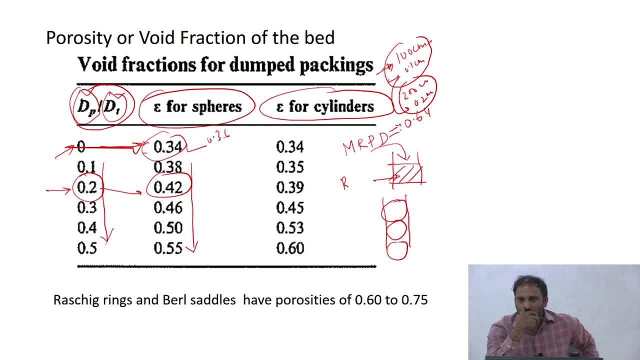 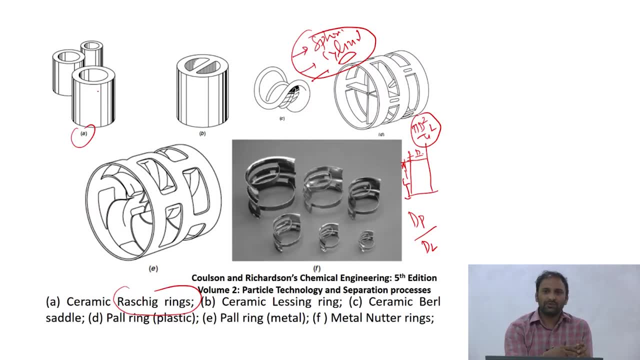 get a similar packing density, ok. So yeah, that is the point. ok, So this is something called as a raschig rings, So you can think about them as you know: hollow cylinders, right, This is something called as a lessing rings, ok. 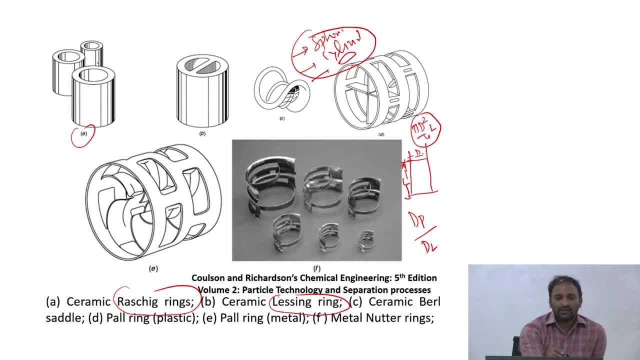 So now, if you So this is something called as a lessing rings. ok, So now, if you take, you look at. So, for example, if I look at this and this, right, in terms of the shape they are very similar, but only thing is in between, I basically have another, you know. 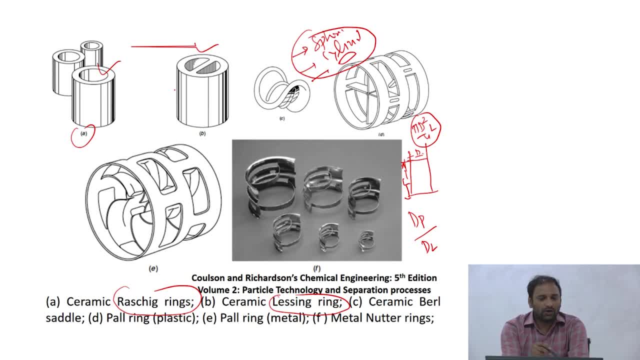 basically a kind of a rectangular, this thing right. So now, if I look at, compare these two, this would definitely offer me a, you know, much more solid surface that is available for any contact right. If I look at this, in this case, the fact that you know I have an- 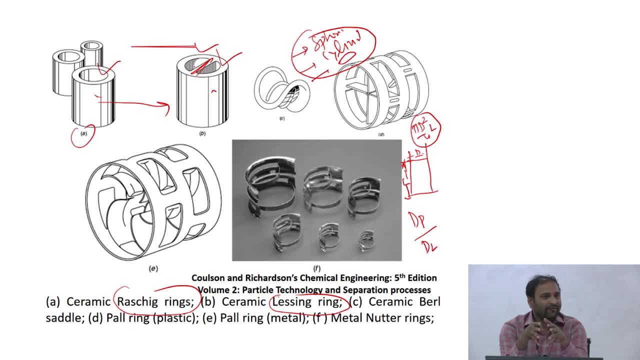 additional. you know region there, So I basically have more solid surface available for any operation that I want to do. So people have using raschig rings, lessing ring, this something called as a burl saddle- ok, something called as a burl saddles- ok. And this is what is called as a Paul ring. this is P A L L ring. 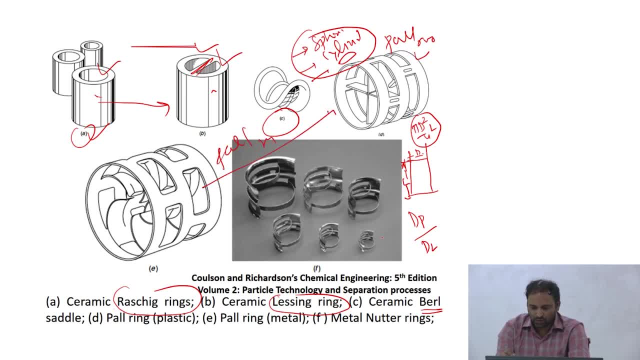 these two are Paul rings, right, And this is one something called as a nutter ring: N U T T E R. ok, This is a nutter ring, So this is a nutter ring, So this is a nutter ring. 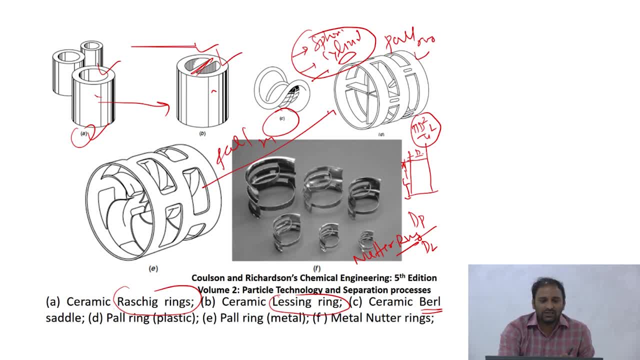 These are different names that people have. you know these are used. these are all industrially used packings of different shapes And, as you can clearly see, you know it is becoming more complex shape, like if you go from A to F, for example, the shape becomes much more. 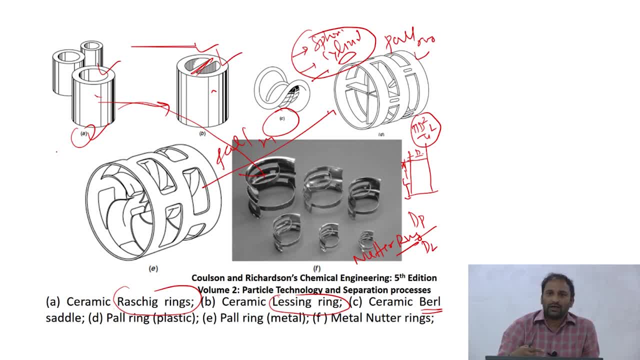 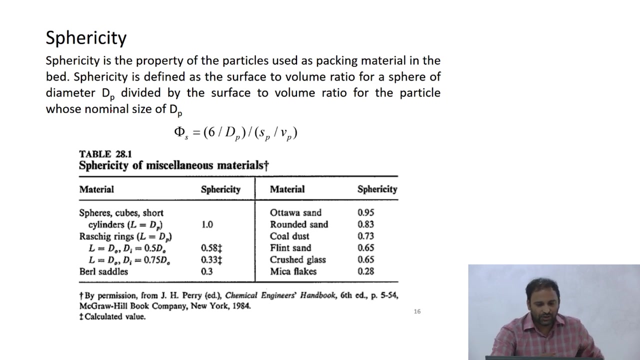 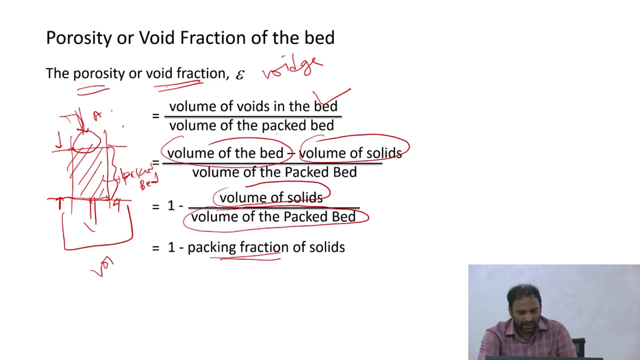 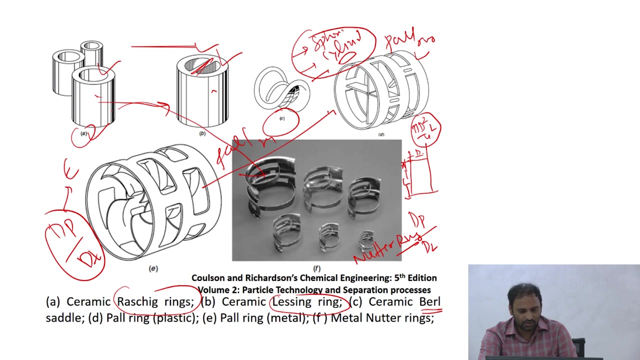 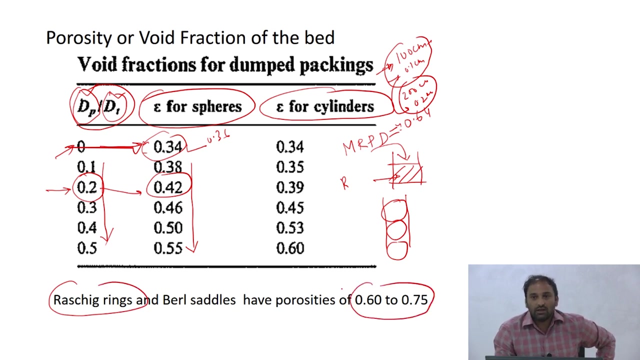 complicated, right, And the reason you know is that you know that will again help you in you know playing with your. you know solid, you know fluid surface. you know areas- right, I mean this range, but now compare it with you know spheres, for example. you see, for 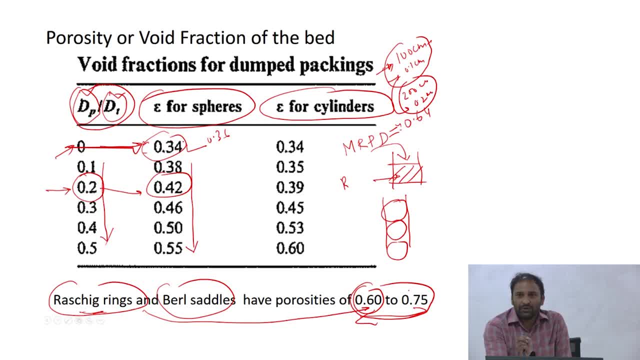 the case of spheres, if I really take a very small diameter particles, ok, The porosity that I can have is about 0.34, even if I increase the, if I, if I play with the, this dimension ok, I can maximum I can go is up to 0.55, but, however, if you use different shaped in, 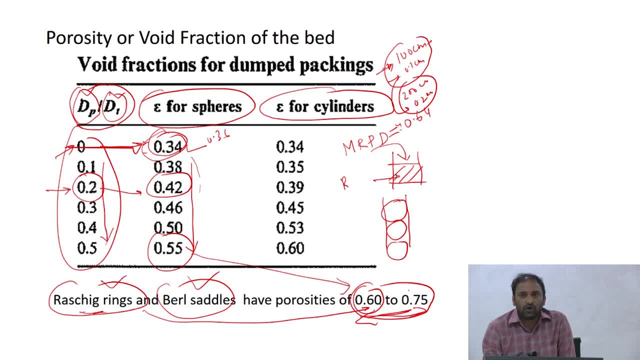 a packing material. I can see that. you know, basically there is a more porosity right, And more porosity would be good for, you know, a better Efficiency of the operation or a better fluid. you know particle contact. yeah, So these are the raschig rings and the ball saddles of the shapes. So basically, if you 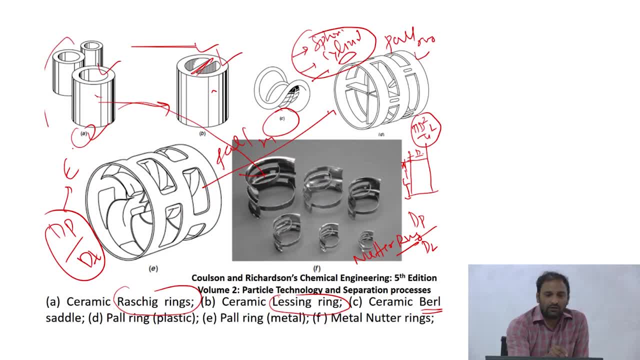 go back here. right, this is your raschig ring. ok, this is your ball saddles, Correct, yeah, correct, yeah. So what you do is when you, when you make a packed bed- right, as I said, packed bed is basically a column filled with a particle- right Now, the particular 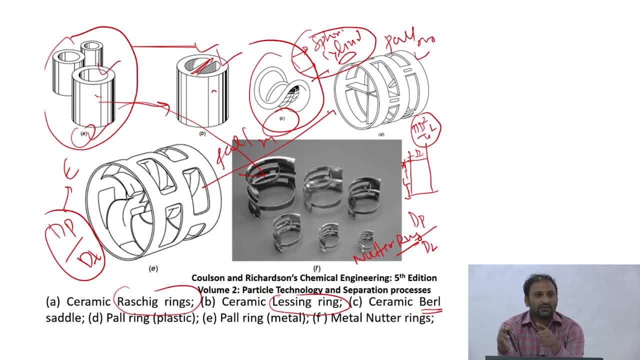 sphere. Now the particles. I have a freedom of choosing whatever particle that I am working with. Of course, if somebody is working with, like say, a catalytic reactor, I would have to use a packing material that is a catalyst that you want to use for a particular reaction. 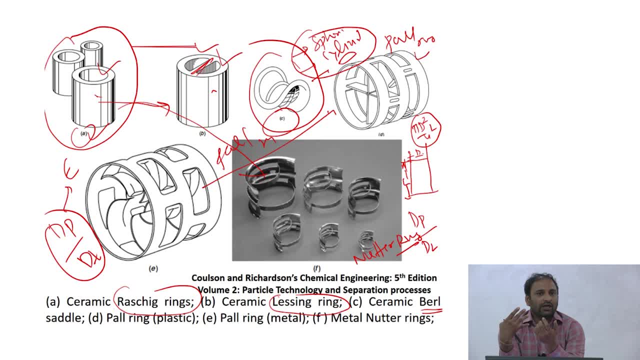 right, or if I, if the, if the, if I want to basically use an inert packing, ok. That means you know these are not past participating in any reaction. if the objective is only to improve the liquid fluid, you know liquid gas contact, for example- ok. 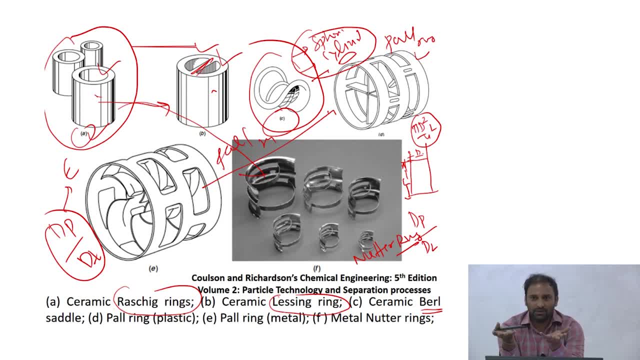 I would like to have a a much more surface area that is available right or more porosity, for example. So in such cases, what you do is you use one of these packing materials. you know, I can basically play with the, a porosity. that will also help you in playing regulating the pressure. 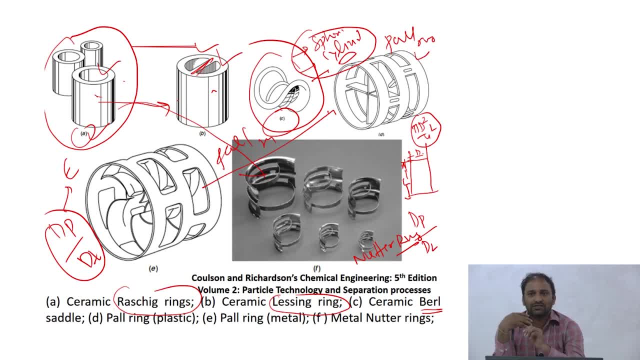 drop through the packed bed, ok. plus, it will also hensure a efficiency increase in the efficiency of the operation, ok. So any other questions, Ways of doing this? so I said you can play with the particle and the and the column diameters and I can play with the porosity. I can play with different objects of different shapes. 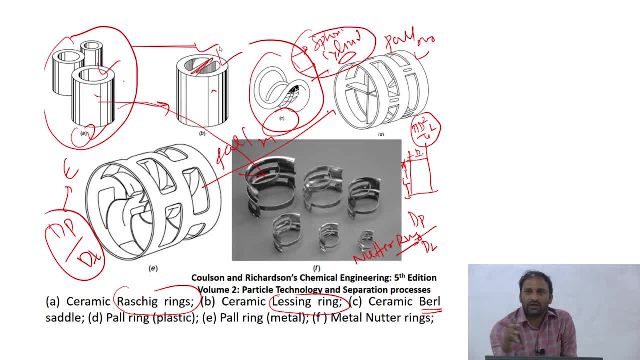 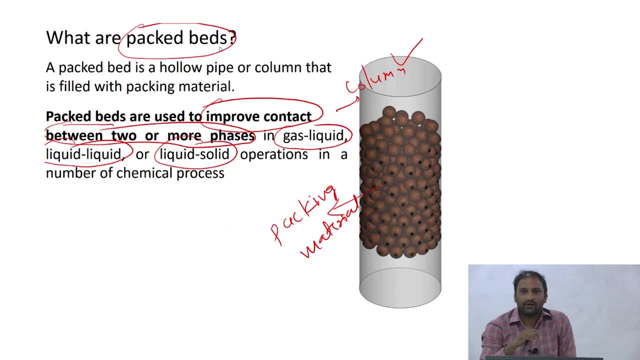 or you know different. you know complex geometries and I can play with epsilon that way. Any other? yeah, you have a question. So these are basically. let me go back. ok, Here I showed that. you know, in this image it looks like a sphere, right, right, I have. 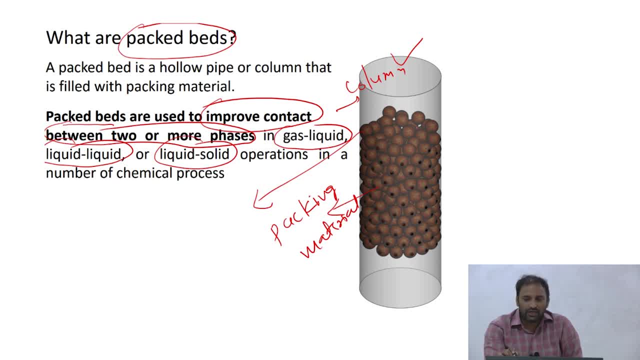 put on a spherical particle in the column. ok, instead of that, I can use a raschig ring right. right, I can use a lessing ring right. So that was actually your column like that, but with a right right, I can use that, I can. 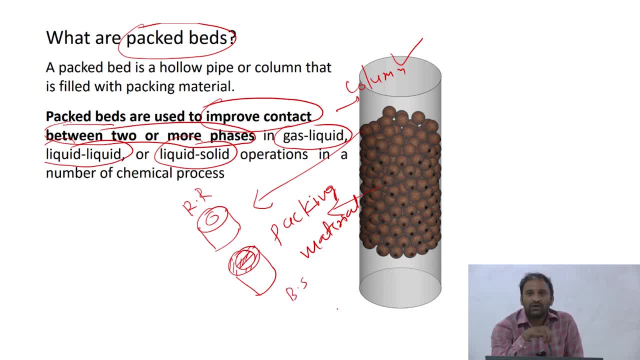 use ball saddles, Any of the packing you know shape that you saw, I can actually replace that. this spherical particle that you are seeing here, I can replace with any of these things and that will help me in regulating your epsilon. ok, that will help me in regulating the solid fluid. you. 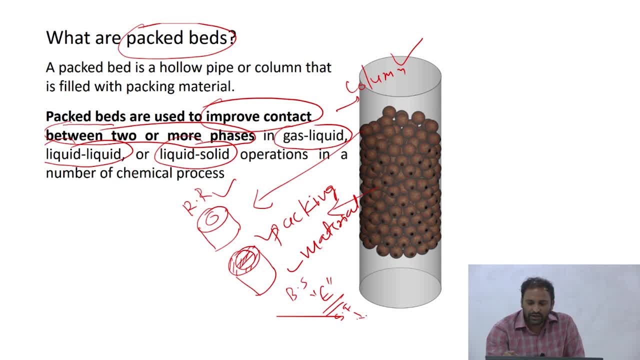 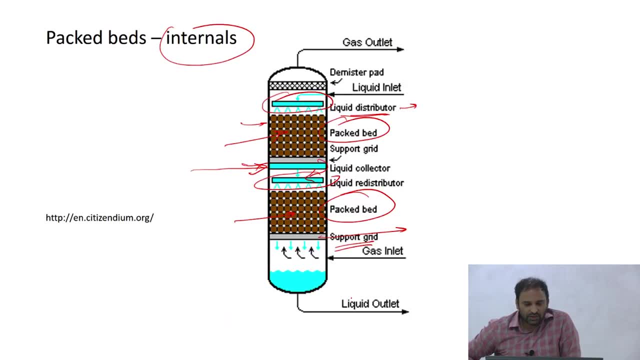 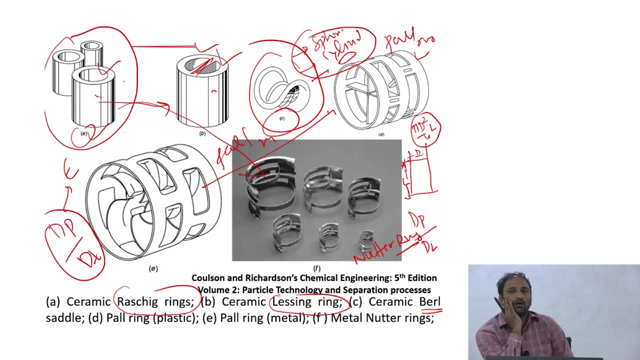 know contact, ok, and it will also help me in regulating the efficiency of the operation. ok, yeah, So any other methods of Any other methods of regulating epsilon? No, no, yeah, no, no. when you say more porosity, ok, what does it mean to you? So, essentially, the volume that is available for the fluid. 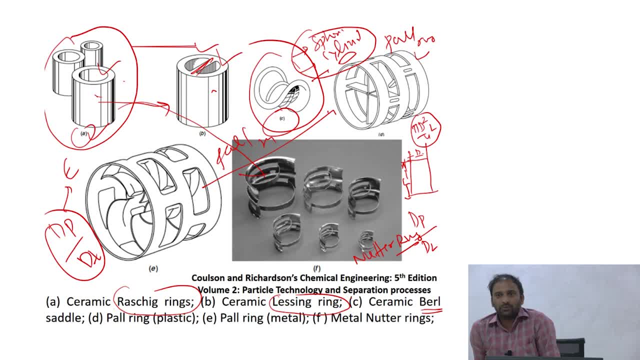 is more right Now, when the volume that is available for the liquid is more. if I say, then I am using a liquid gas operation. ok, You know, of course, the part of this. you know the fractional void A that is available. there will be liquid and the gas right The more. 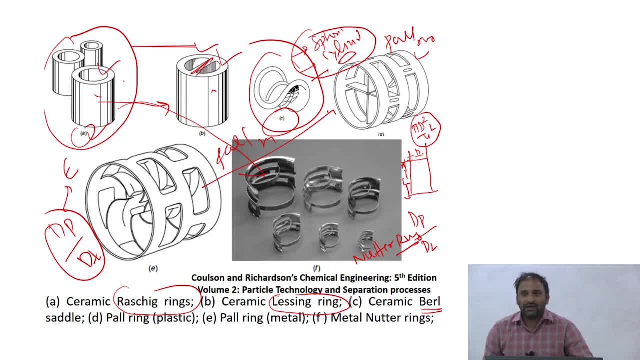 the volume that is available, there is more contact between the gas and the liquid right. in that sense, you know, regulating porosity is a way of. I mean, people go for more porosity because you know, if you want to really improve the efficiency of the operation, I would definitely. 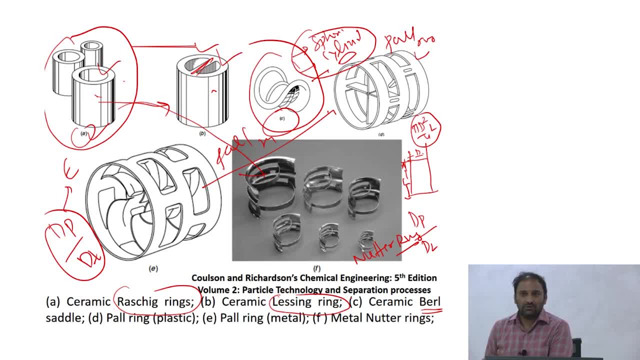 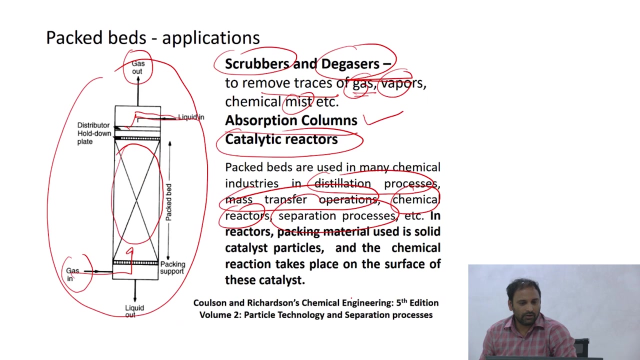 like to have more porous, correct? No, like I give an example where if I have a pipe, right, ok, I let the liquid Liquid and the gas flow through the column. ok, When people talk about this two phase flow in the columns people talk about let me just go back. ok, When you talk about two. 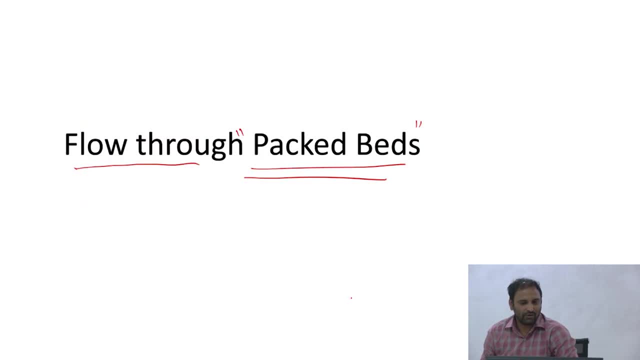 phase flow. let me just go back here. ok, So when you talk about two phase flow to, for example, say that you know I have a pipe, ok, I want to have a liquid one. or say liquid one. or say let us say fluid one and fluid two. that is flowing through the column, ok, through. 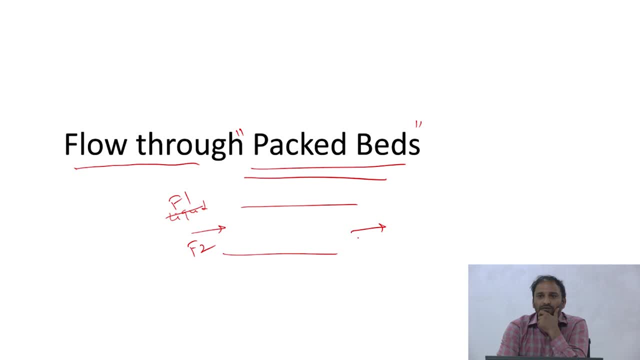 the pipe, for example. ok, What do you think would be the? how would the flow look like? or let us say two immiscible liquids, liquid one, liquid two. they are two immiscible, say, but I would like to have a proper contact with contact between the two. 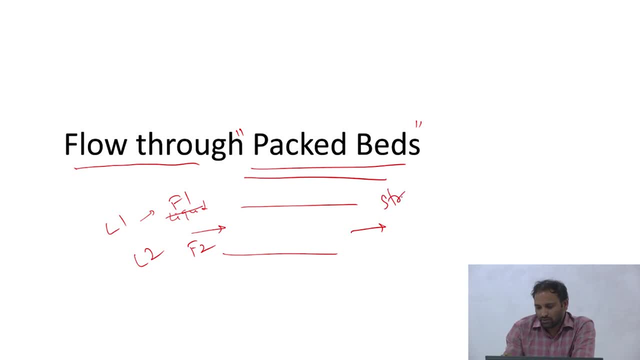 But people talk about something called a stratified flow, in which I have liquid one flowing above, In which, In which- So liquid one flowing above, maybe, and liquid two flowing below depends on the density of the fluid. So there is a two right. that is one way of doing think about it, The other 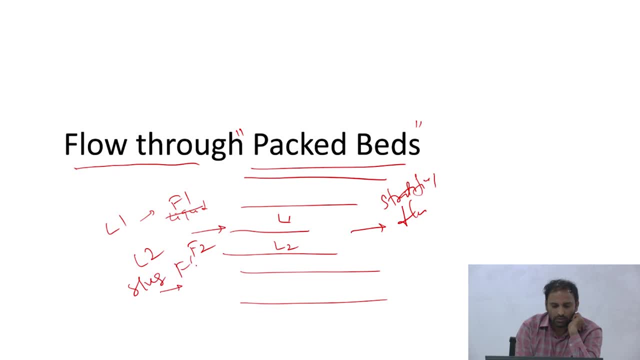 way of doing this would be: people talk about slug flow, ok, In which you have, you know your liquid one could be here and you know liquid two will be outside right. this is liquid one, ok, So it basically goes this right. Now, if you look at these two cases, the liquid- 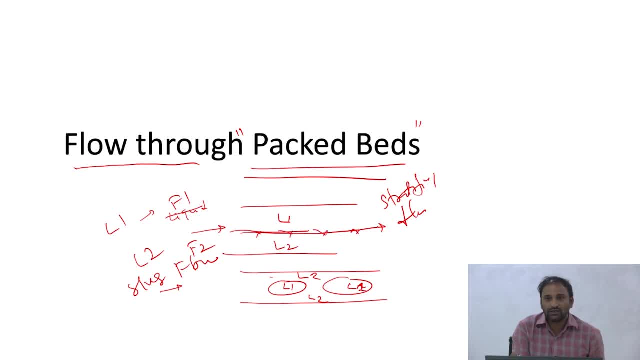 liquid contact actually is happens here. right, you are only at the interfaces when the liquid contact. So if I look at this slug flow, there is a little bit better contact because you know I am, I am able to break the stream into. you know, maybe you know these slugs, ok, but however, 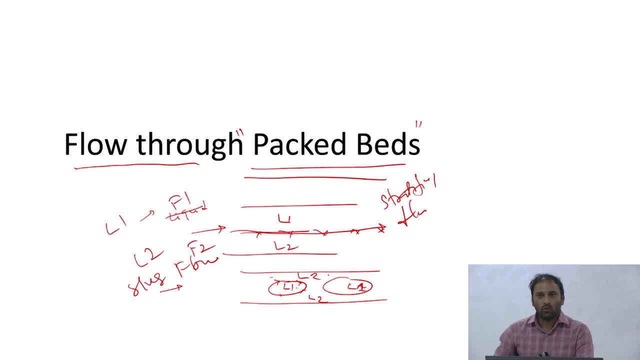 you know your liquid, liquid contact is still limited. Now, if I you know what is the best way to ensure that you know, you know there is a larger, you know kind of a interaction between the two fluids. ok, When I say interaction, not the, you know the interaction in terms. 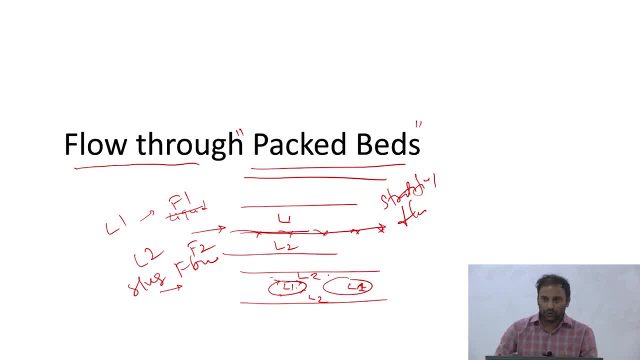 of the molecular interactions, but I would like to have a proper contact between the two. ok, But the best way of doing this would be, you know, using these devices where you know you can ensure that you know there is a better impact. So then, less porosity. 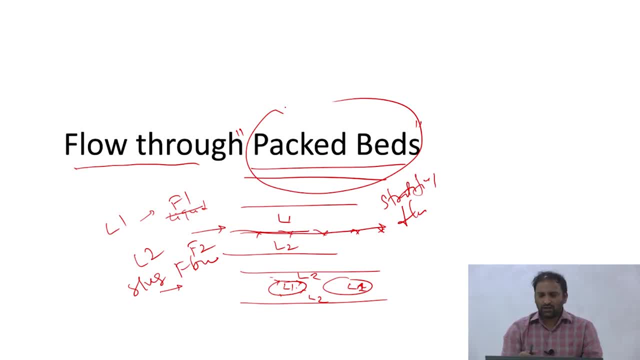 Why do you say: the less porosity, more the break. So I mean, see I you cannot think of the. So, in this case, are you talking about porosity? in this case, why would you talk about porosity in this case? Because, because, if I look at this, your entire column is filled. 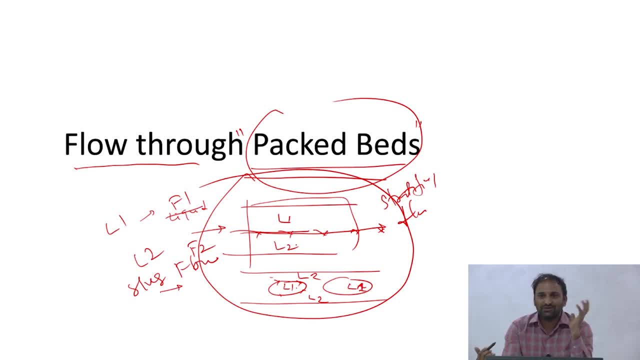 with the liquid. So in that sense, you know there is no, No pores as such. right, I would not say, would you really call it as break the fluids? no, I mean, you know, you see, you have just like you know, just like a liquid flowing through a column. you should imagine that you know there is also a liquid. 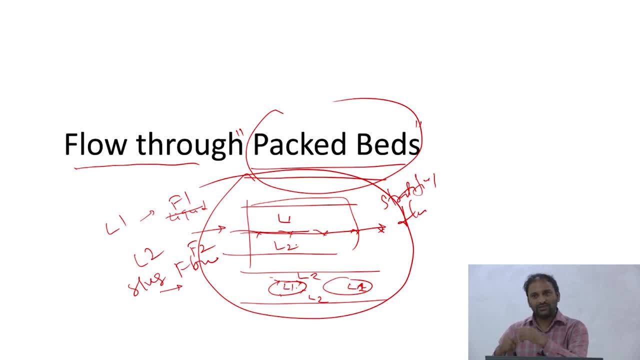 flowing through a bed of solids. ok, There are channels available for the liquid to flow through. ok, Now, as it flows through. if I have one or two different fluids, ok, and you know it will have a, you know it will basically give more chance for the liquids to interact. 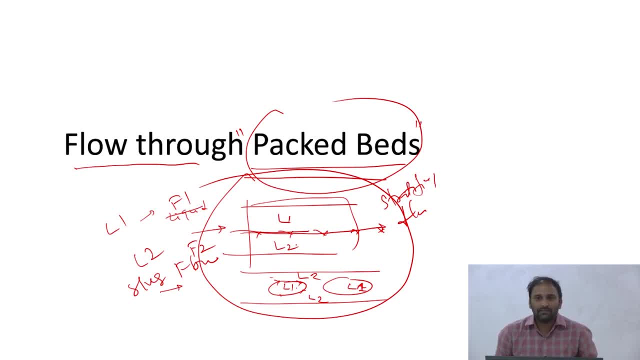 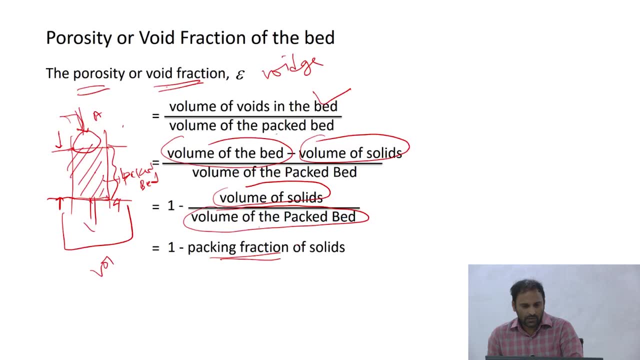 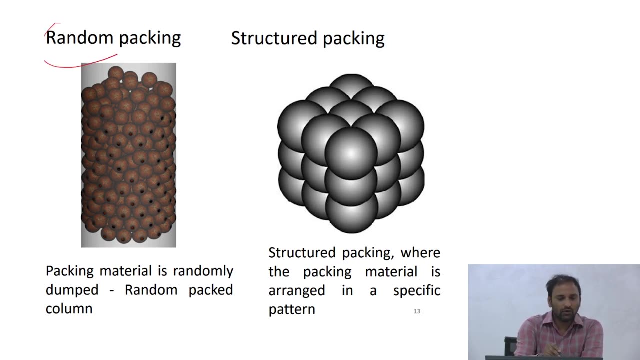 let it put put in that that way. yeah, yeah, ok. So the other way of doing this would be looking at something called as a random packing versus structured packing. ok, So if you take a column, you just pour your- you know- particles into the column they pack in. 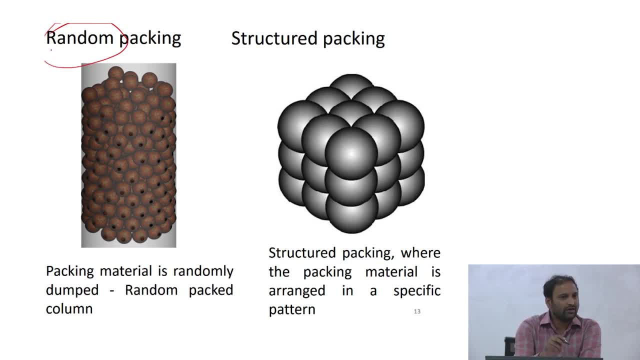 a particular way And typically, if you again there are ways, there are actually kind of prescription as to how you should fill the packing into your you know column, ok, And if you follow some procedures you will basically end up with a truly random packing ok And other way of. 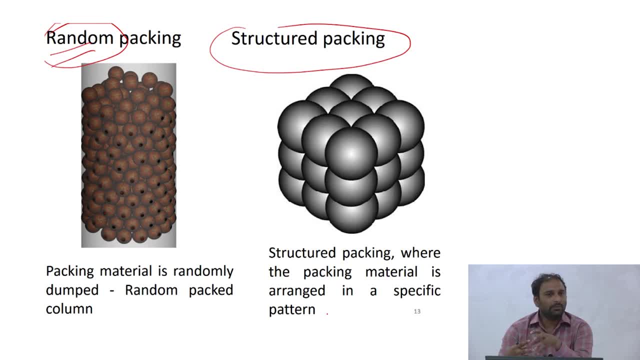 doing this would be what is called as a structured packing, in which I have a some predefined way in which, you know, the solid material is basically arranged. ok, So I am basically, you know, showing you the random packing of spherical particles here and the structured packing of spherical particles here, And, as you can clearly see that you know in this, 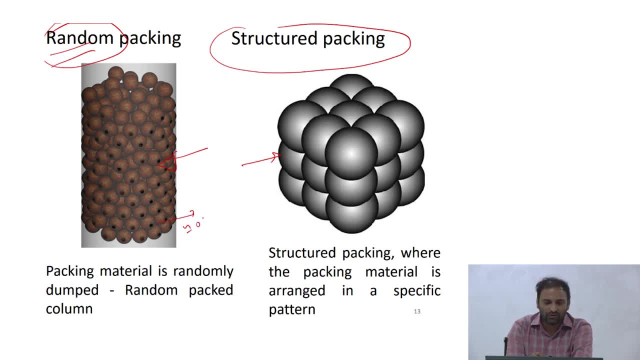 case that typically the porosities that you can achieve would be of the order of 0.36 and if you do a, you know a random packing here. But however, if you look at this case, you know packing fashion is more. if I assume a particular kind of packing, you know right. 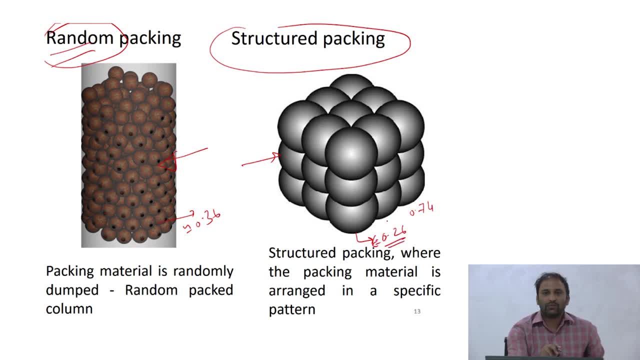 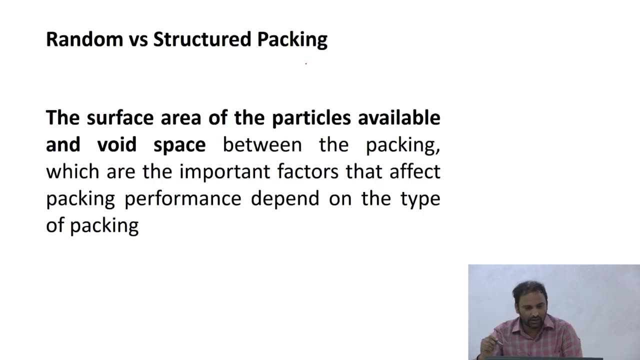 your porosity is going to be right, So. so basically, the other way of you know playing with your you know porosity is go for random versus structured packing. People typically do not use particles and then do a structured packing. So what is done in the in the ok? 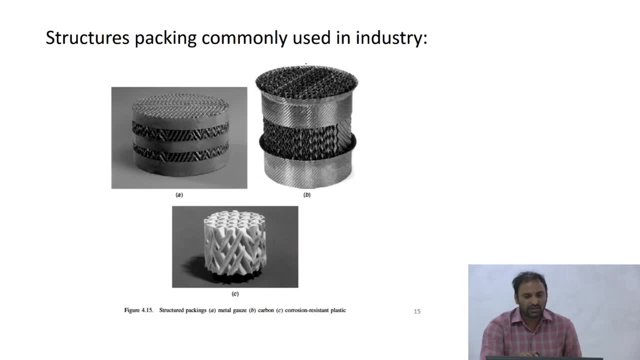 So I will come back to this point. So this, these are some kind of structured packing that people use. So these are what the what you have is. you basically have structure which are either made of some polymer or it could be made up some of some metal, in which you 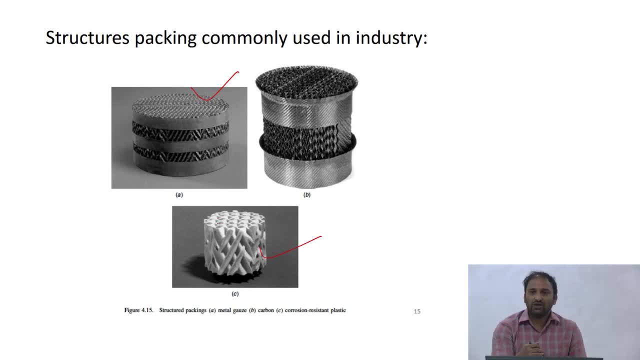 basically. So your, if you look at this pictures, right, the solid part, right, the solid material that make the packed bed- there is a you know particular way in which it is constructed, right, ok, And that that forms the solid in the packed bed and whatever pores that you see here, right, 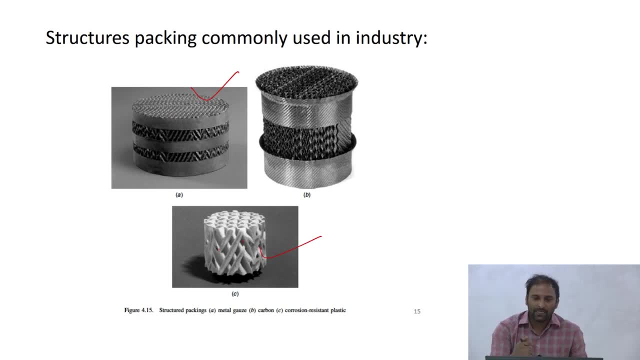 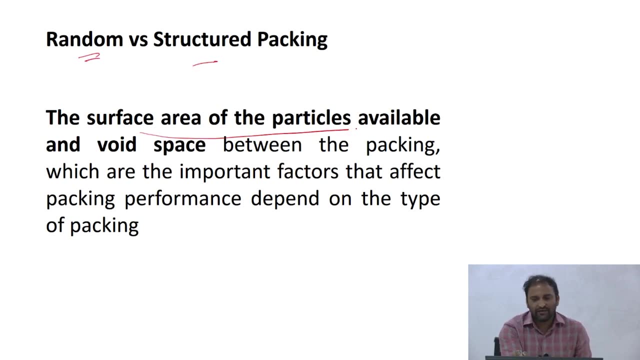 there is a pore spaces through which the liquid basically pores through. ok, So, and the idea of using- going for random versus structure packing is that you know, the surface area available for the liquid and the void space I can basically manipulate right, like just the point that I made earlier, So I can basically play with the voidage. 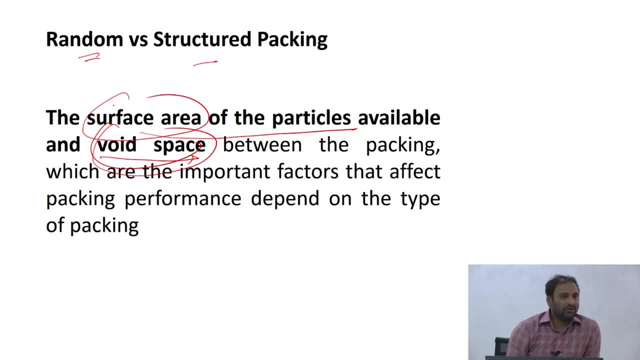 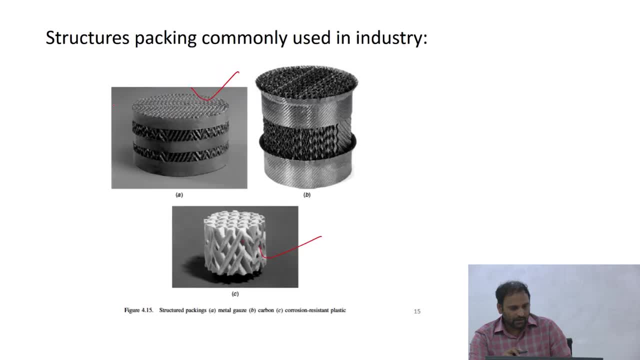 plus. also, I can play with the surface area that is available for the fluid-fluid contact by using these devices. ok, So we have defined this parameter called sphericity and it turns out- you know, if you look at when you are going to talk about this- delta p, which is a pressure. 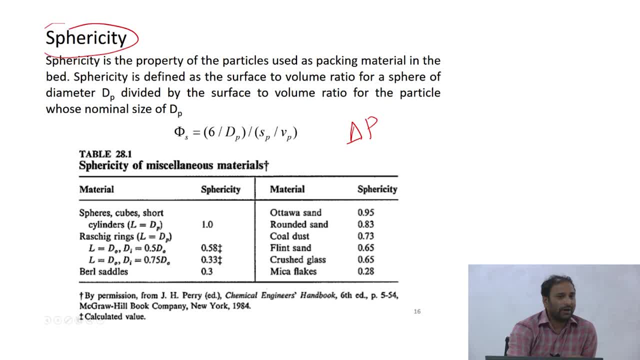 drop Through the packed bed, the sphericity also becomes important parameter. ok, We have defined what it is already. it is defined as sp by v? p of a sp by v p of a sphere divided by sp by v? p of the particle right and sp by v? p for the sphere is 6 by d? p and sp by v. 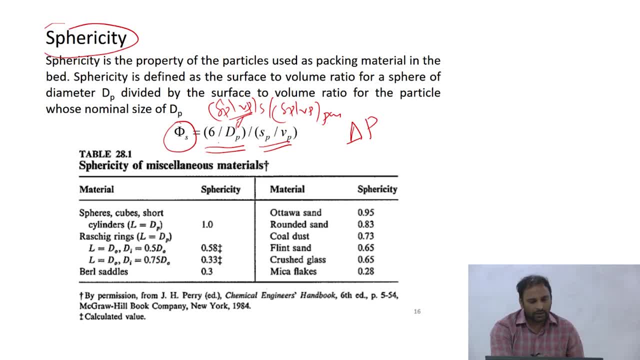 p, that is for the particle, that is your sphericity. And and if you see here, if you look at the spherical particles, or you know, or, or cubes, or short cylinders, your sphericity is 1. ok, And if you go for raschig rings, this is l is equal to d p. that is your, you know your. 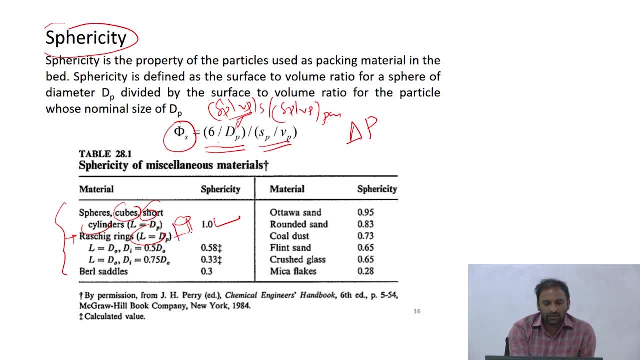 your, if you have this raschig rings, right, that is your cylindrical kind of thing. So that is your length and that is your d p right. So if l is equal to d p, if it is a short cylinder, sorry, raschig ring. So if you, I can play with these dimensions, I can actually 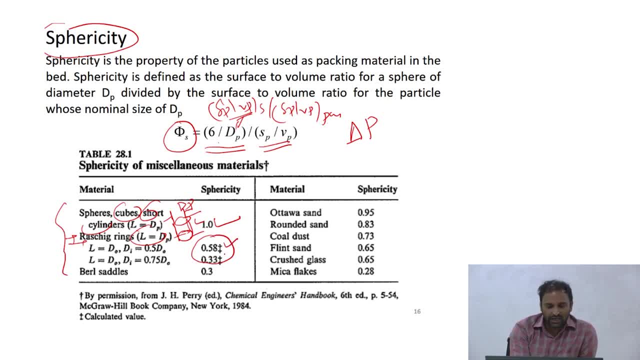 play with the, The, The porosity right, 0.53 in one, 5, 8 in one case, you know, 0.33, in the other case, Burl saddles typically have a sphericity of 0.3. ok, And these are the, the kind of industrial. 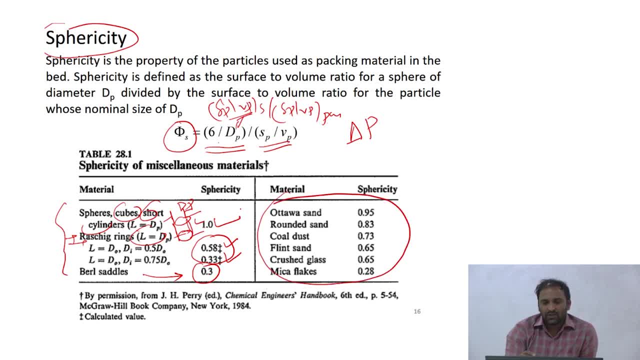 packing that people use and people also work with. for example, you could, you can, have a, a column in which you know you may be working with some kind of sand particles, or you could be working with coal dust, for example. ok, In such case, again, you know your sphericity. 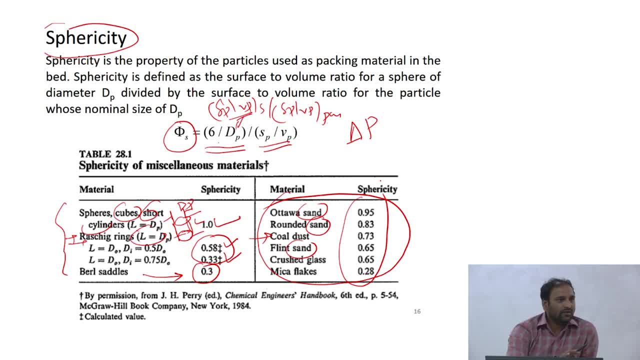 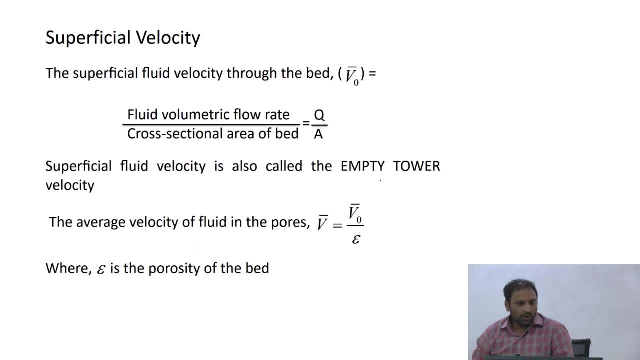 would vary. ok, So there are ways by which, as we discussed in the class, there are ways by which I can basically calculate sphericity, right Other term similar to the multi particle system. there is a concept called superficial velocity, which is basically defined as the volumetric. 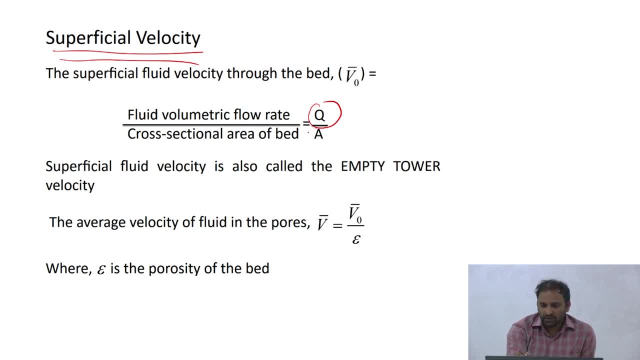 flow rate of the fluid through the column divided by the cross sectional area- that is your q- by a. it is also also called as a empty tower velocity. ok, Superficial velocity is also called as a empty-tower velocity. this is the velocity of the fluid through the column when there is no packing. ok, that is your q. I know if. 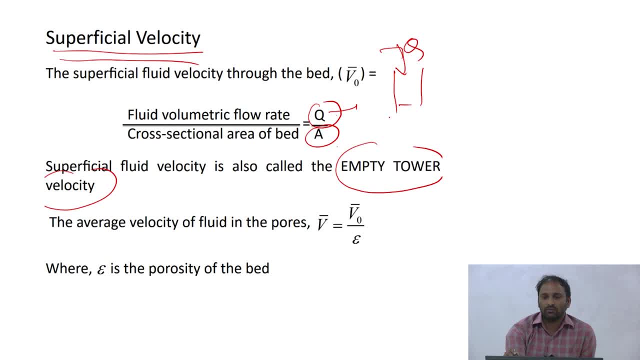 I have a column, if I have a way of measuring what is the flow rate through the column and if I know what is the cross sectional area. that q by a is what gives you the superficial velocity right, also called as a empty-tower velocity, But the average velocity of the 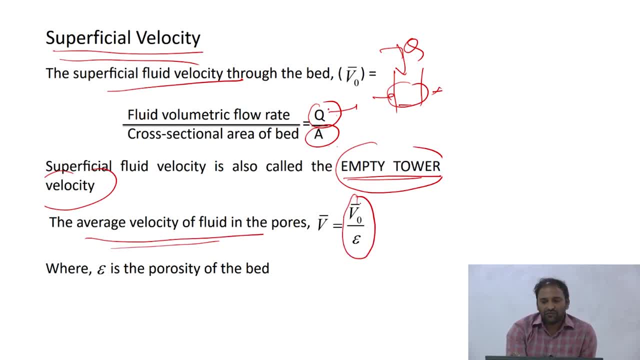 fluid through the pores is basically your. You know, The surface velocity of the fluid through the pores is called as the flow rate of the fluid through the column. And the way I can define velocity, superficial velocity divided by epsilon. right, because epsilon will tell you. 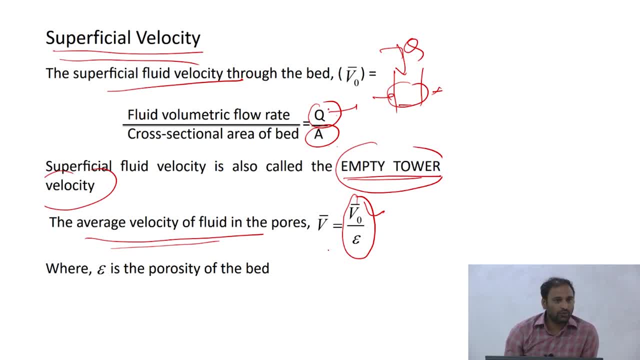 what is the cross section here that is available for the liquid to flow through? right? ok, That is the actual velocity or the average velocity of the fluid through the pores. ok, yeah, So that is about it. I just wanted to briefly introduce you to the concept of packed beds. 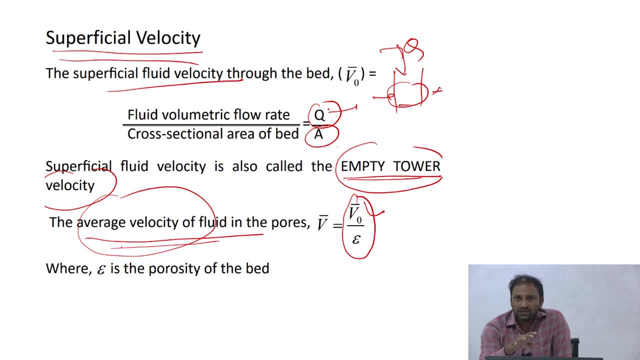 today We have talked about what are packed beds, where are they used. we talked a little bit about packed bed internals, that there is a liquid distributors, liquid collectors. you know, and you know some concepts like that. We defined a few parameters: voidage and the 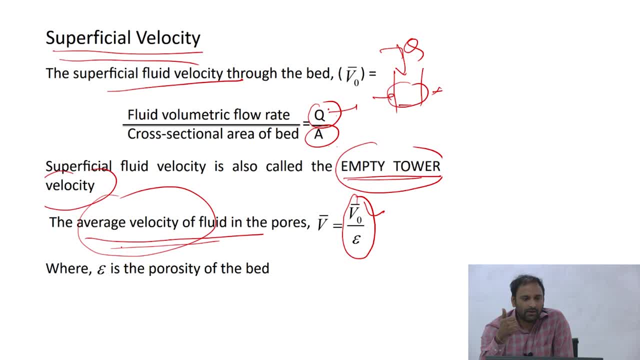 sphericity. we talked a little bit about superficial velocity and we also talked about different types of packing and different types of packing material and water. what are the different methods by which people manipulate your porosities? and you know the fluid solid contact area that is available for the ok. we will stop here. 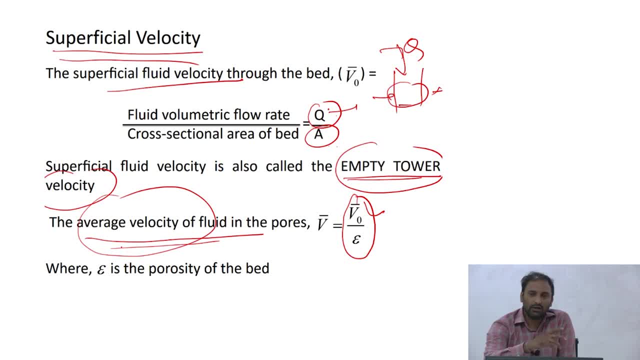 On Monday we will have, we will talk, start a talk. we will start talking a little bit about pressure drop through the bed. ok, we will. what we do is we are going to take the analogy of flow through pipes and you know, we kind of apply that to the flow through.